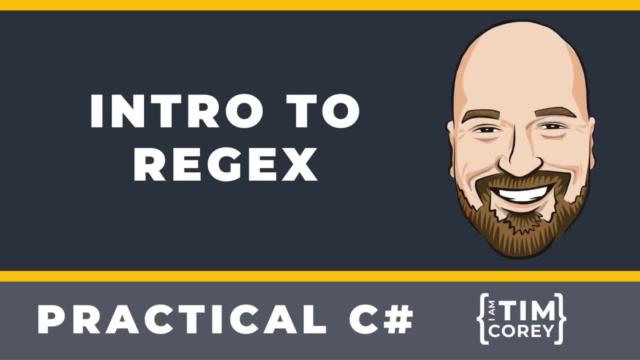 but you'll also be helping to fund my free content so that everyone can have a great education, not just those who can afford it. Okay, let's jump right in. Let's jump right into Visual Studio. We're going to create a new project that's a console. 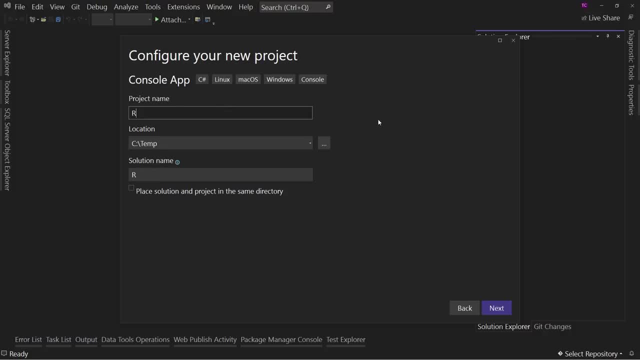 application. So I choose Console App and let's call this Regex Demo. We'll call it Regex Demo App. If you want the source code from today's video- yesnet6- and no, don't check this box. If you want a source code for this video, go in the description of this video and you will see a link. 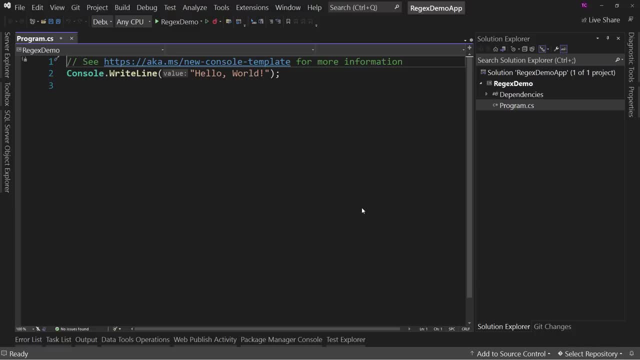 to download it. I'll ask you for your email address. I'll send you an email with the code in it. Okay, So let's start off from scratch, with nothing in here. We're going to start from a blank slate And actually, 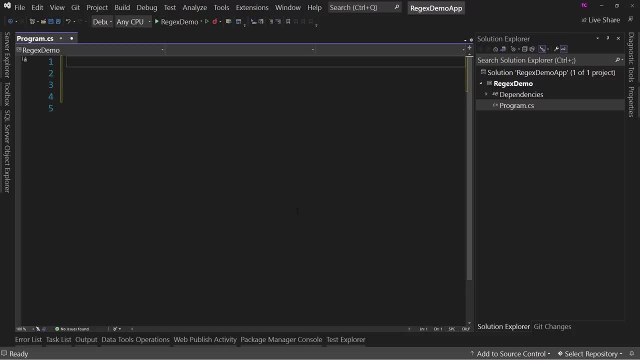 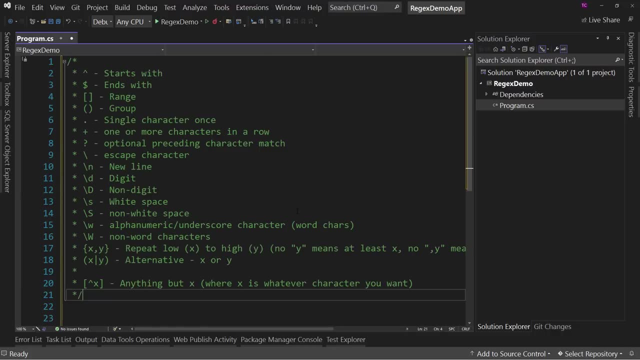 what I'm going to do is I'm going to the very top here, I'm going to paste in a large code comment, And this is a cheat sheet. And I want to start you off with a cheat sheet because regular expressions have a lot of scary looking things in them, But really, if you have this cheat sheet, 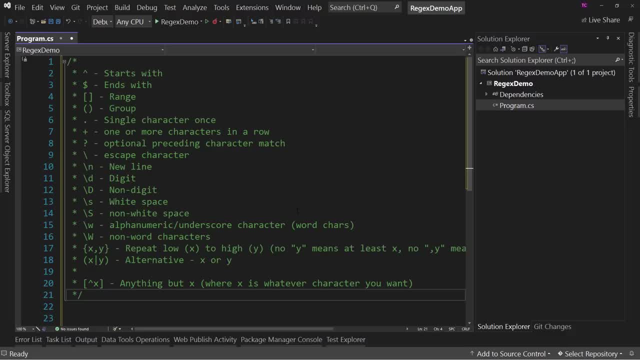 you're pretty much set for building your own or for diagnosing someone else's, Okay, So what we're going to do is go through and start using this cheat sheet. So I'll explain more about each of these pieces in a little bit, But let's start right away with a regular expression Now, in 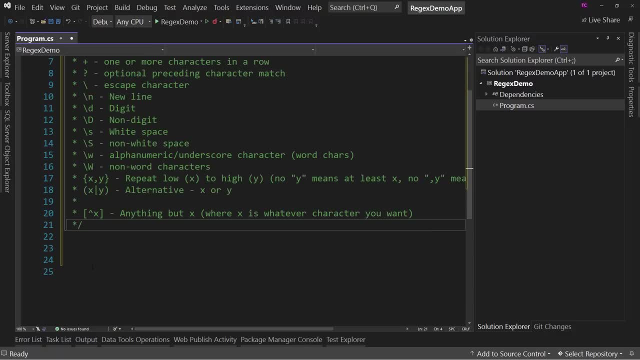 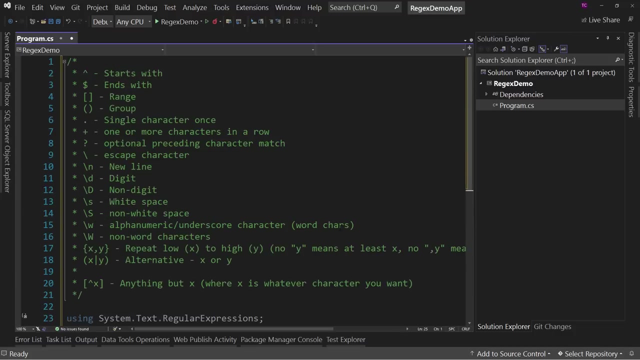 order to have a regular expression, we need to have a using statement. So let's do it right here, underneath our cheat sheet, using systemtextregular expressions. All right, that will allow us to use regular expressions. Now let's talk about what a regular expression is before. 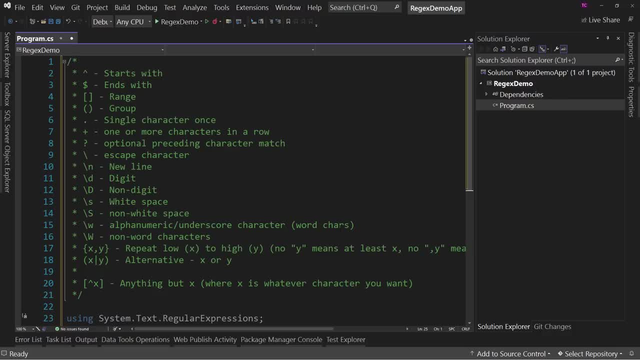 you start seeing them. A regular expression is a thing like a query. So if you were in SQL and you said, Hey, I want to look at this table, but not every record. I want to say where the last name equals code. So if you were in SQL and you said, Hey, I want to look at this table, but not every record. I want to say where the last name equals code. 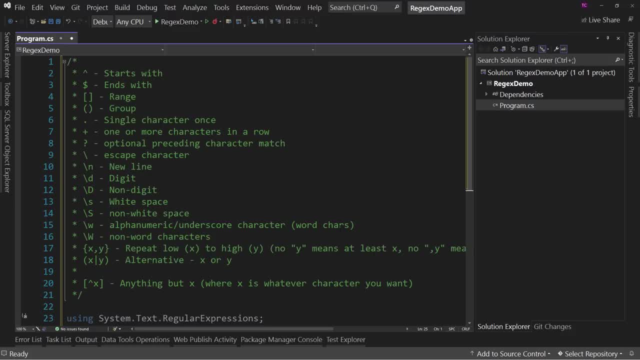 Okay, that would be a query where you kind of filter down the results. Well, a regular expression is kind of like that, in the fact that we say, Hey, I want you to find something. But the cool thing is is it's not just as simple as I want you to find. the last name equals Corey. 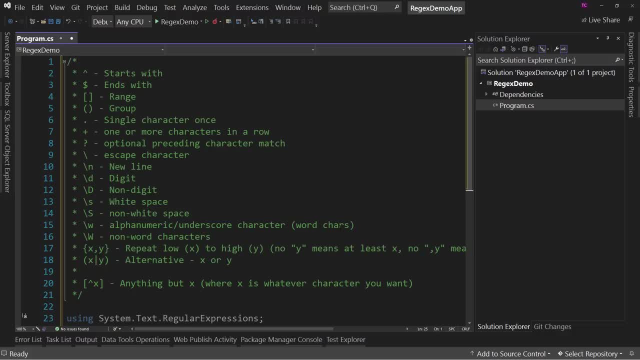 It's. I want you to search this entire text file and find me every phone number in it. What's the phone number? Don't know, Could be different, And we're going to do that by the end of this video. So that kind of thing is a lot more complicated. You can't say Hey, does this. 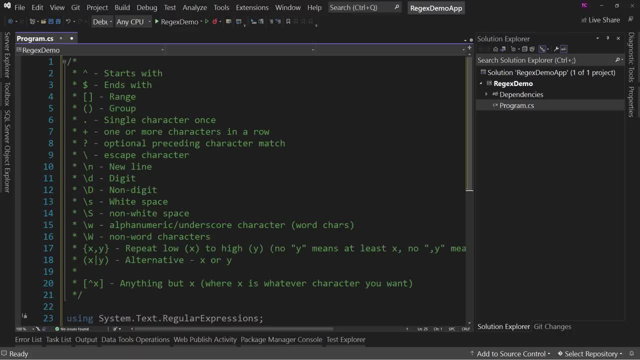 line of text equal this phone number. Well, if you don't know the phone number you're looking for, how would you know? And that's where regular expressions come in. Regular expressions are pattern matching. They say: Okay, you've defined a pattern, Now let me go find the match for that. 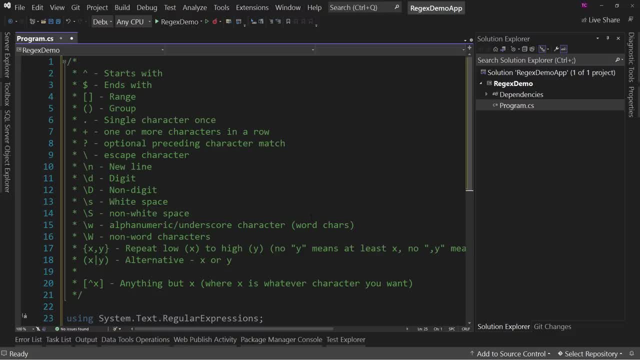 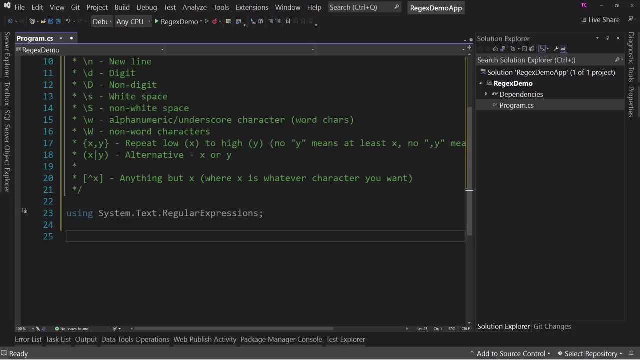 pattern. So let's see us, And we're going to start by starting small and simple and then kind of grow until we get to that more complex- find every phone number in a 5,000 line text file, Okay, So let's start with something simple. We're just going to say: let's start with a pattern. 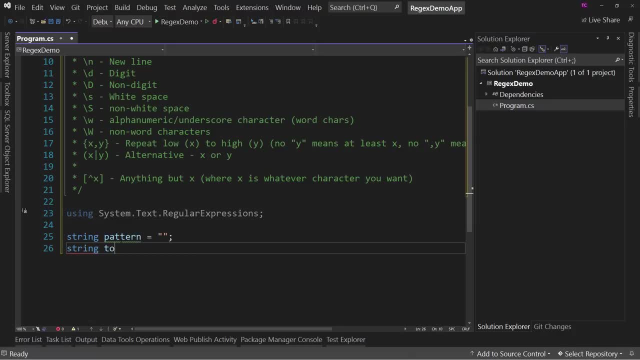 and then we're going to have a to search string. Okay, So the pattern is: here's the pattern to look for and then here's a string to search it in. All right, So let's, let's do this, Let's create a pattern that says: Hey, I'm going to look for Tim, Okay, 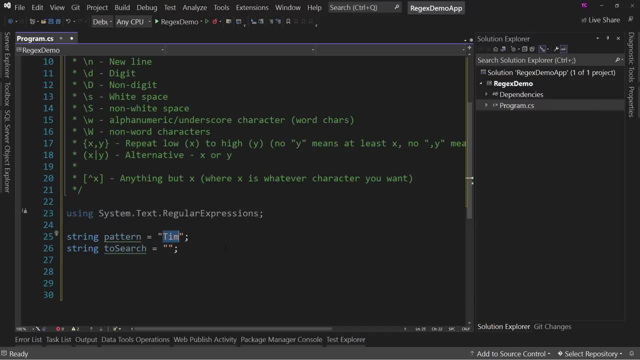 So we're going to look for Tim. That's a pattern. Now that's just three characters, but that is technically, or can be a regular expression. It's a pattern to look for. It's a very specific pattern, but it's a pattern to look for. So if I were to say, Tim Corey. 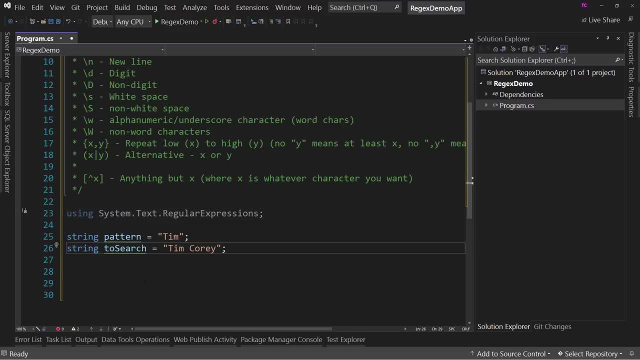 I'm going to look for Tim, which is Tim, and then Apple's going to look for Tim. Okay, It's going to find. in fact, let's do this. Let's wait on the, the cert to search string per minute, And we're going to search a number of different ones all at once because it'd be faster. 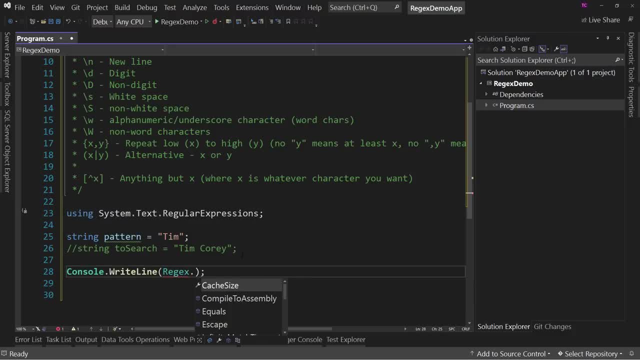 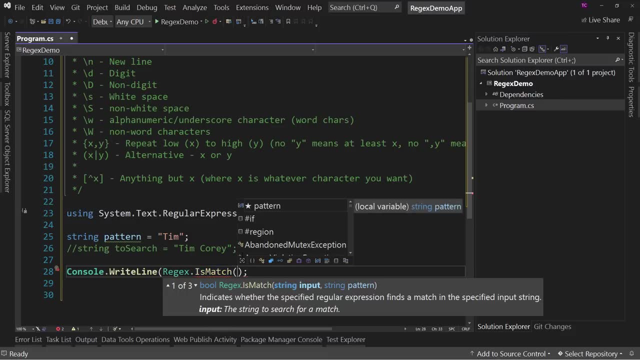 So let's do console right line And we're going to say right in here: regex dot is match. We're looking for a match. It's going to ask for two things on input, a pattern. Okay, So the input is tim corey and the pattern is our pattern we're looking for. so we're going to do is say hey. 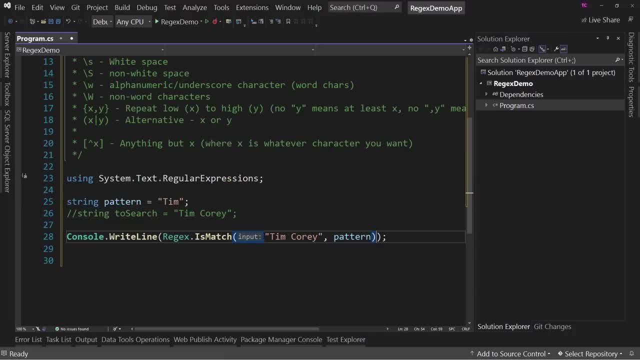 um, we actually are missing a paren at the end. we're going to say in this expression we're saying: hey, is this pattern, which is tim, is that found in this string? yes or no, true or false? and we're gonna get back a true or false and we're saying: console right line here. so let's say: um, 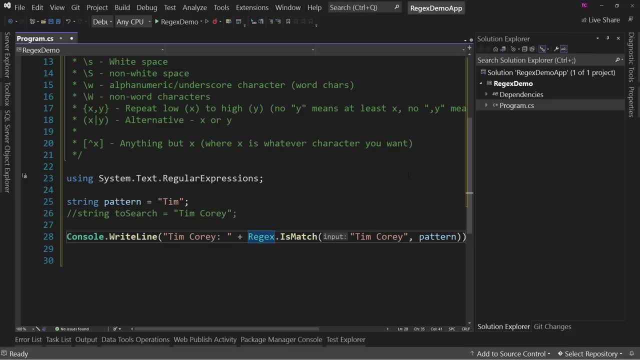 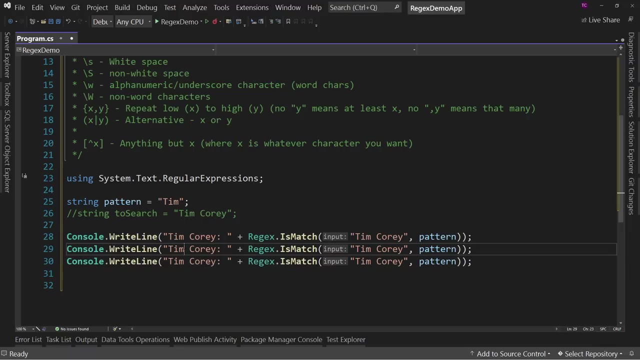 really simple, all right. so we're getting super simple here. we're saying, hey, this console run is going to say tim corey. true, we just found tim in tim corey, hopefully. but let's copy this and do a couple more times and throw it some curveballs. 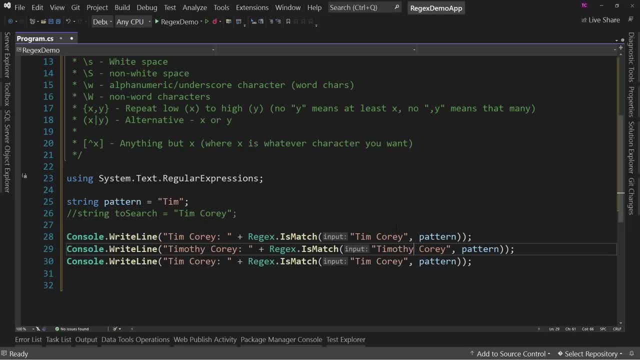 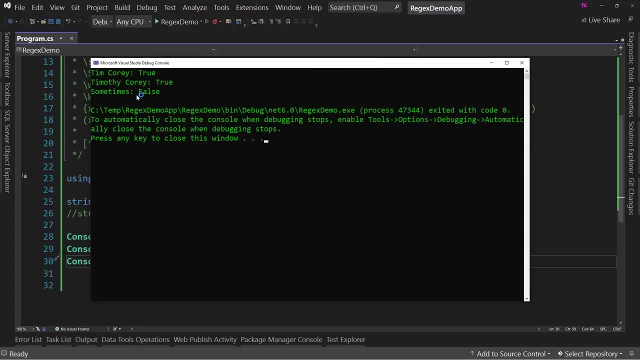 timothy corey. that's actually my name, timothy. now, that's cool, but what about this? you see the tim there sometimes. okay, so we're gonna find out if it's in sometimes, let's run this we've got. is tim corey true? timothy corey- true, sometimes false. okay, so i didn't find the tim. 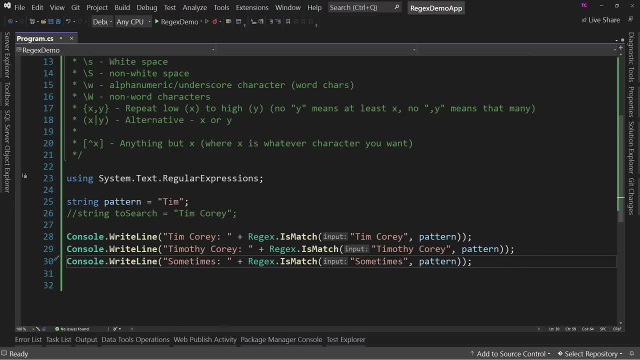 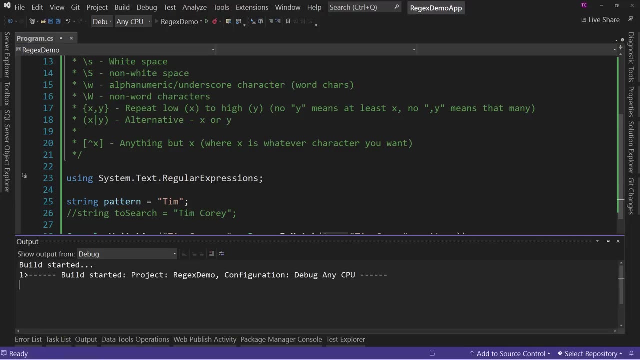 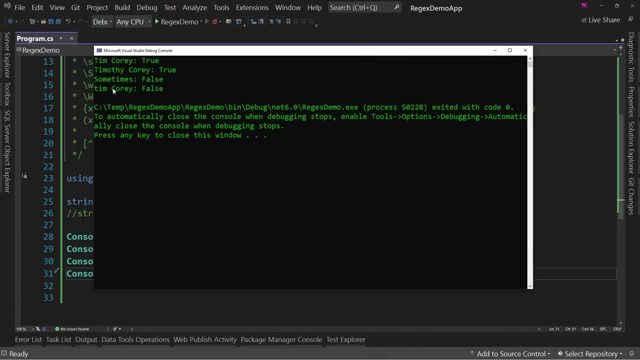 in sometimes. well, why is that? well, he's a capital t. in fact, if i changed this, let's actually add another one here. um, let's add another one like this at the bottom, and we're going to say lowercase t. if i did that, we get lowercase tim corey false. even though it's separated out it, it should be found right, no. 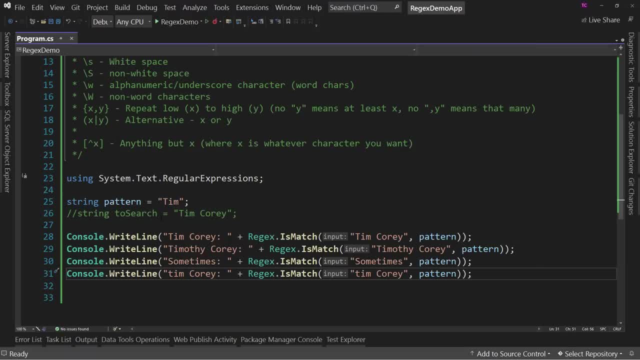 because it's case sensitive. now you can make a regular expression not case sensitive, but that's not usually ideal. so instead, one of the things we can do is we can say this: now: if you go up here to your chart, we see that this is a range, all right. 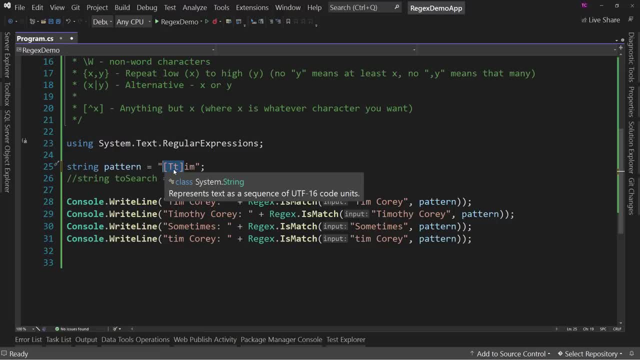 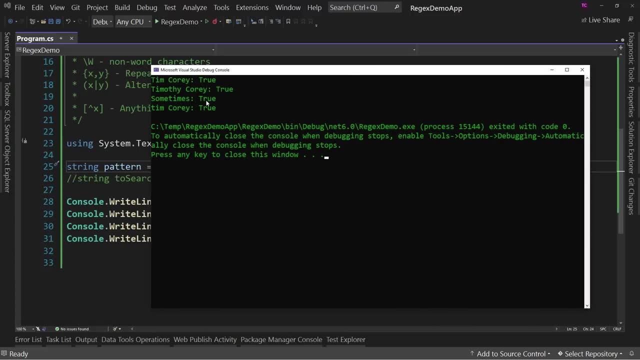 so i have now said either capital t or lowercase t, all right, and if we run this again, we'll see that all four of them are true, including sometimes in. so instead, one of the things we can do is we can. sometimes we've found team in the middle, so we have found matches in all four of these strengths. 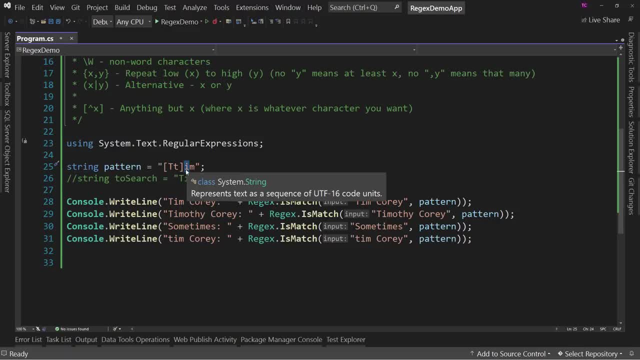 now, we wouldn't want to do that with every letter. i mean technically could, but that'd be kind of a pain. so we could say right here: um, our options is ignore case. all right, we can do that. like i said, it's usually not the best, but we could ignore case here. in that case we have the tim like this: 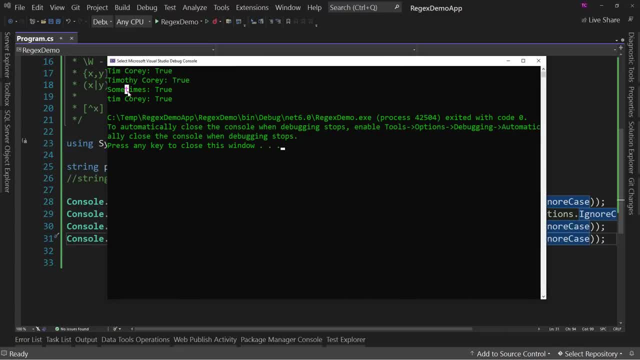 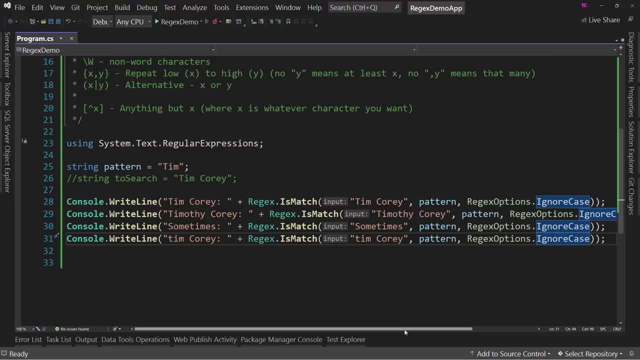 and you find all four are true, even though this is a lowercase t and so is this okay. so you can ignore case again, not my preferred, but you can do that all right. next up, let's make this a little hard to get rid of, because it's a little hard to get rid of, because it's a little hard to get rid of. 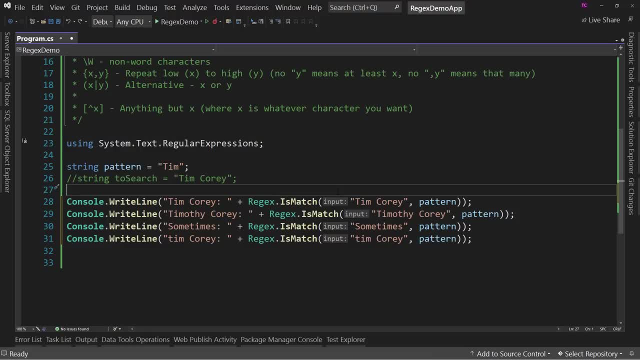 all right, next up, let's make this a little hard to get rid of. all right, next up, let's make this a little harder. so what if we said that we're looking for the name tim, only tim, as a name meaning capital t lowercase? i am with. 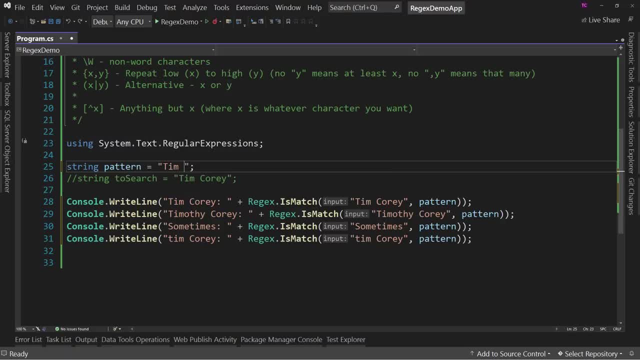 with spaces on both sides. so we're really looking for something like this, but that's not going to work necessarily. so let's just ask for tim to start and let's run this and see if any of them apply, and we know the bottom two won't. 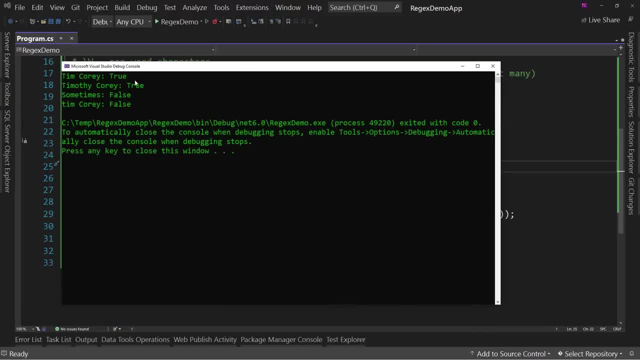 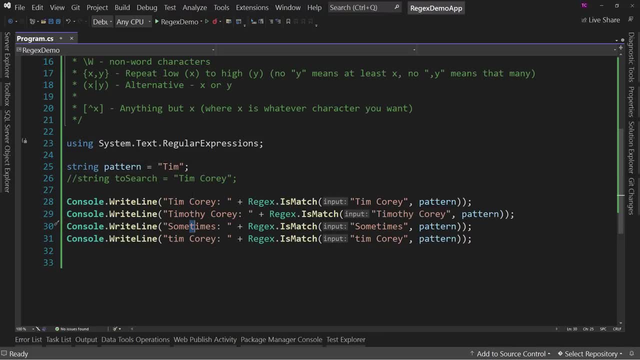 and see if any of them apply, and we know the bottom two won't. we have two true and true and false and false right now, with just tim. right, because these two fail, because lowercase t. okay, but what if we wanted to say that we wanted this? let's start. let's start with simple, let's start with. it has to start with tim. 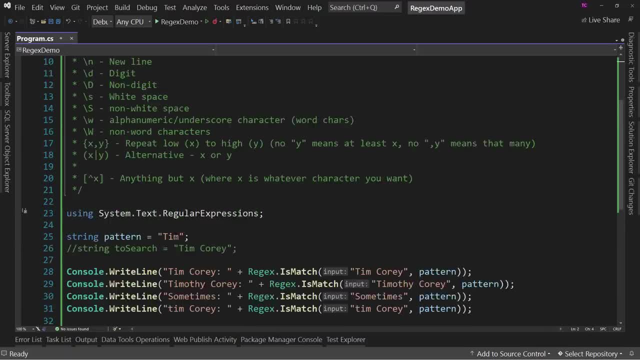 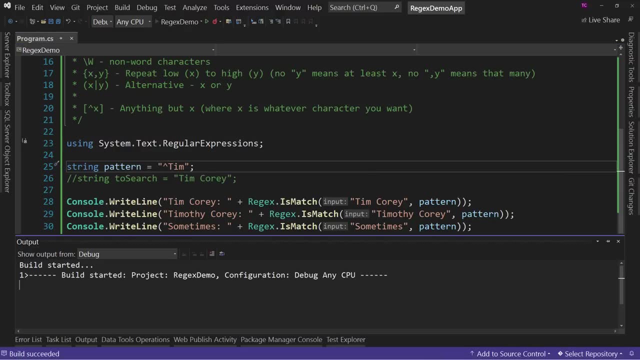 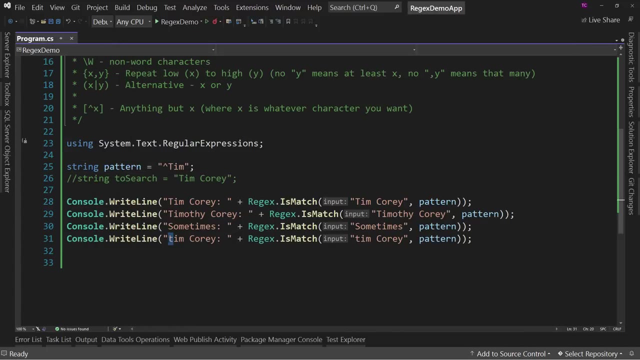 well, come back up here, starts with. so we say: starts with tim. well, come back up here, starts with. so we say: starts with tim. And you run this and we get true, true, false, false. Still, let's change this up a little bit and say: I am Tim Corey. 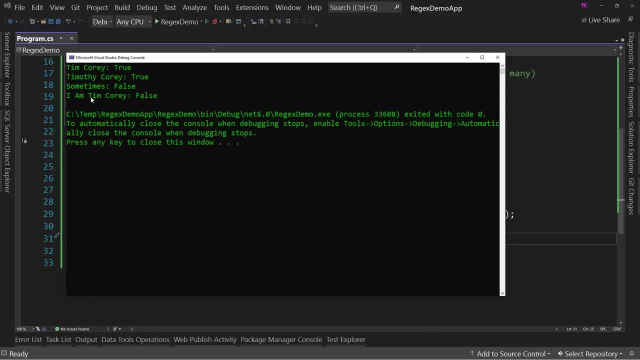 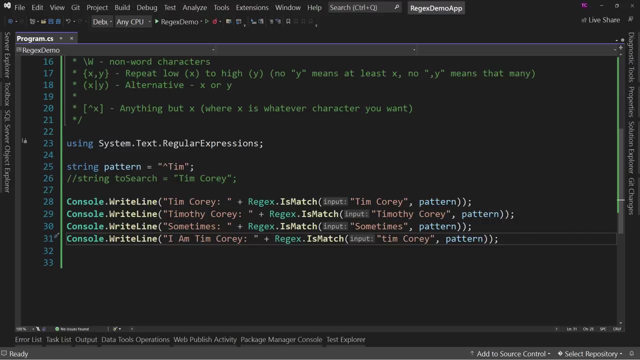 True, true, false, false, Because even though capital T- lowercase I am- is in the list, it's not starting with Tim. Now remember, I say for well, if it's looking for the name Tim, which we could say well. 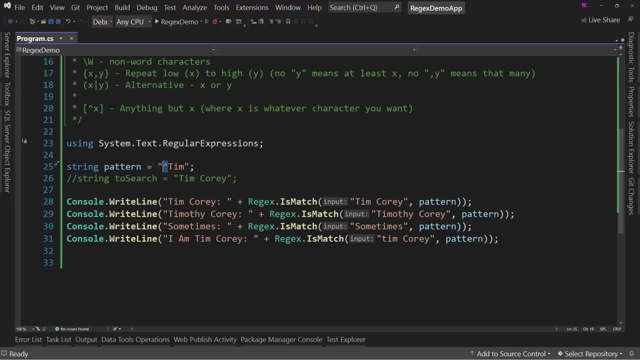 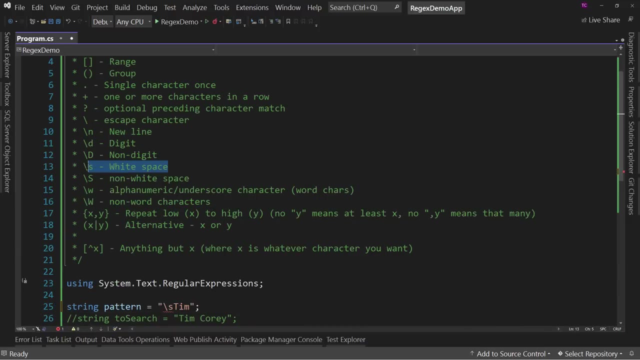 I want this to be, Tim. surrounded by spaces like this, one is to see that it's a word. So I could do this. or I could say slash S If we look up here, oops, wrong, slash, slash S. We look right here: white space. 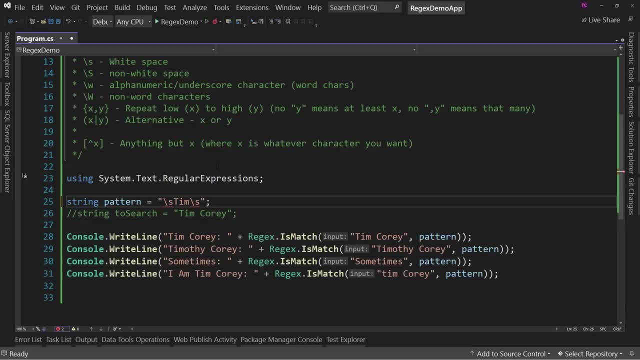 So I could say slash, Slash, S again at the end for white space at the end. but notice, we get the red squigglies: unrecognized escape sequence. That's because for regular expressions we have to use the string literal character, the at symbol in front of it, because otherwise it says actually you're, you're trying to. 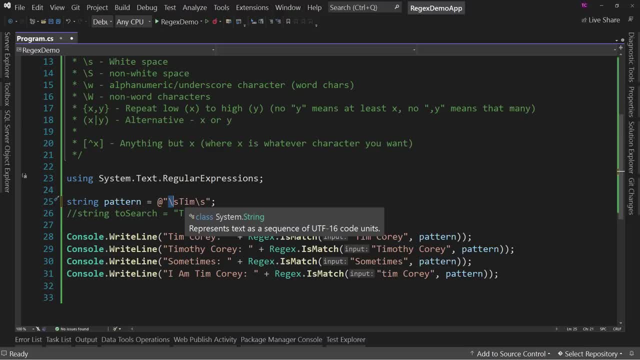 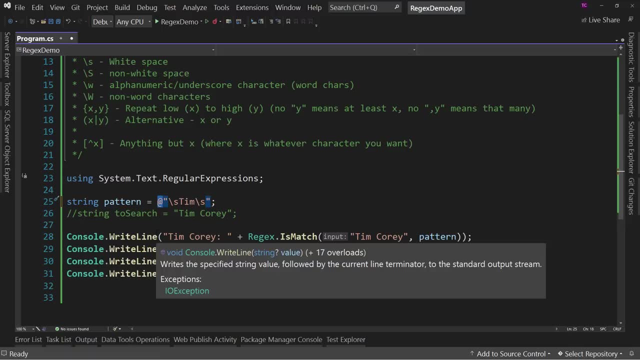 escape an S, but I don't know what an escape S is. It's not thinking regular expressions, It's thinking of the C sharp escape sequences. So we want to say this is a, a, a string literal me. take this literally as it is. 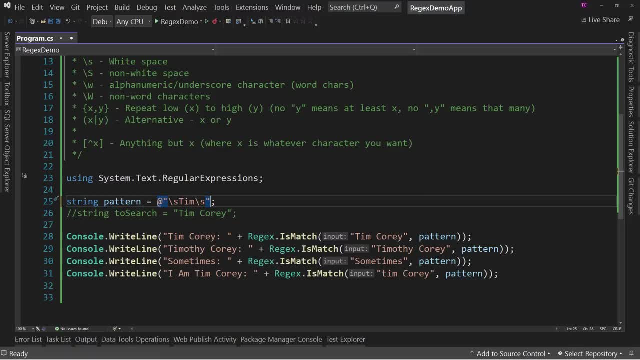 There's not anything special in here. Now, for real expressions, these are escape characters, but they're escape character for regular expressions, not for C sharp. So that's why this tells it: for C sharp There's no re. there's no escape characters here for regular expressions. 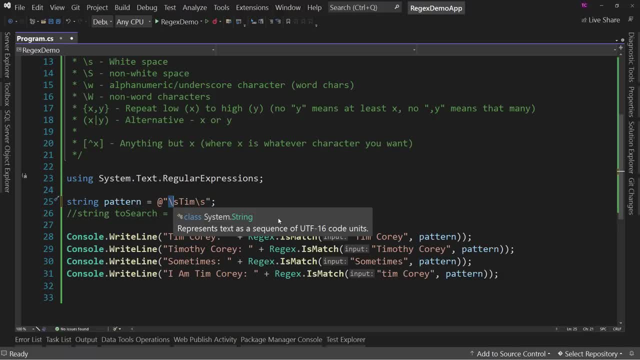 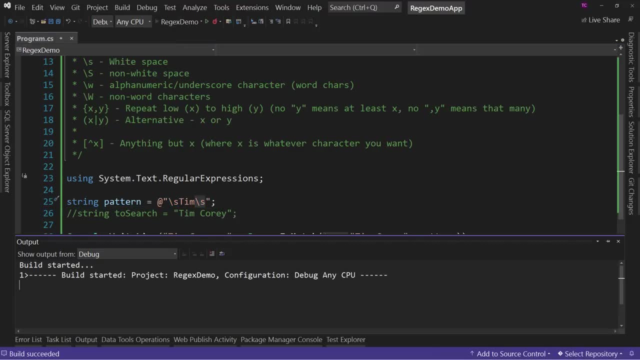 When it processes it as a pattern, it'll say, oh, that's an escape character. So, yes, it's a little bit different. Okay. So now we're saying: is there a space on both sides of Tim? If you run this again, we'll now see false for all four of them. 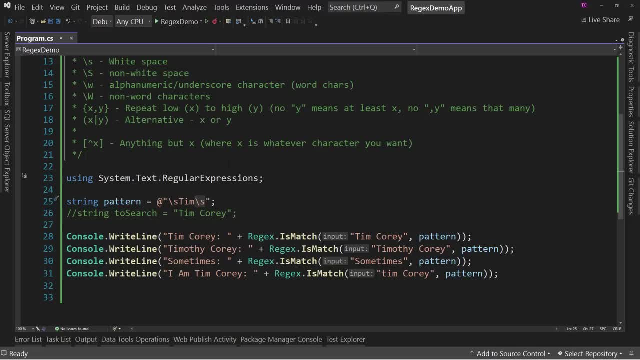 Well, why is that? Well, that's because I've been modifying the wrong thing, Whoops. This is why it's not great to have duplication in place. I didn't modify that, So let's do this again. um, because I messed this up and it might've worked. 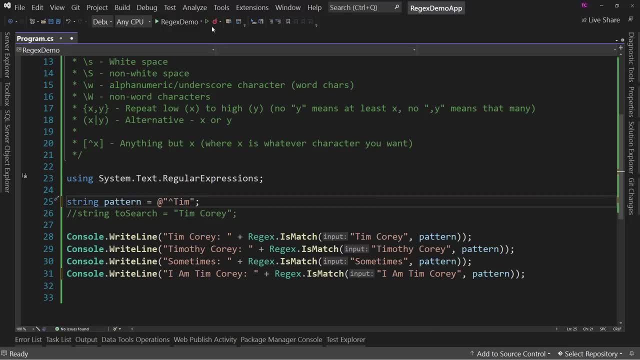 It's not going to. but it might've worked if I had said starts with No, it's still says false. Okay, It doesn't start with it, It's in the middle there. Okay, Now let's look for the space at the beginning and end. 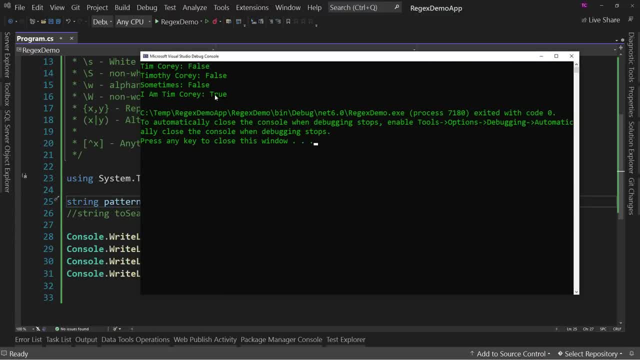 And you run this and we get true. So I am Tim, Corey is true, because we've got Tim standing alone. So we've- we've said yes, the name Tim, not Timothy, not Timmy, not any other variant of Tim, and not sometimes with Tim in the middle, but Tim. 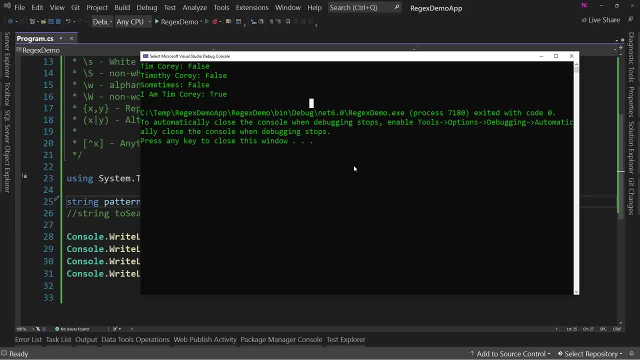 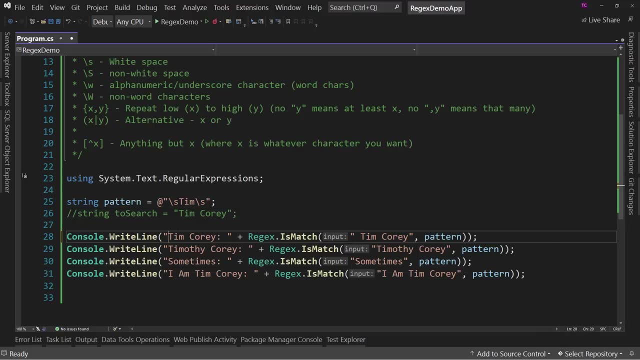 Okay, We're looking for the name Tim and he found it in the last one, but that's really not complete, because we found it in the first one too, but there's not a space before Tim. In fact, if we would change this, there is a space before Tim, or run this. 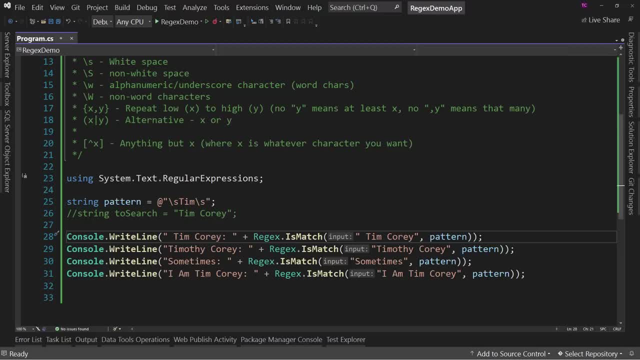 Now, that's true, but it's it's not right. I mean, we, we shouldn't be doing that. So how do you find where Tim is at the beginning? So we found Tim in the middle, with spaces on both sides. 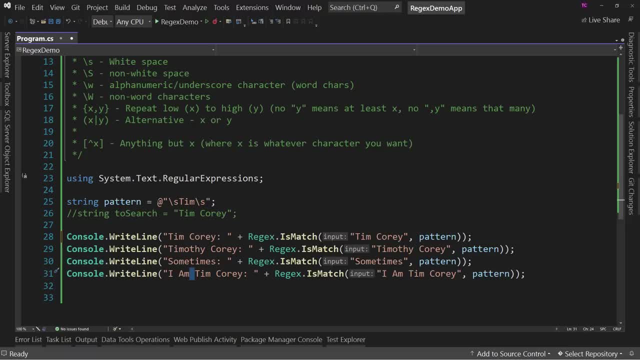 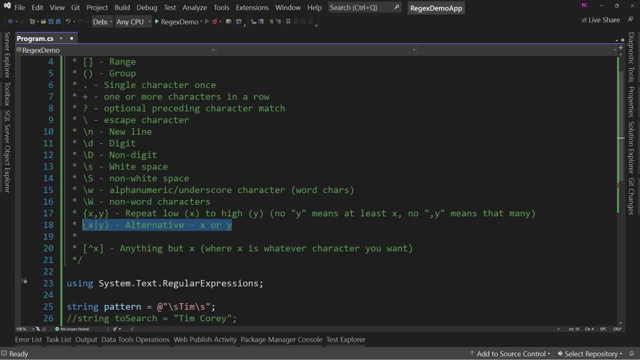 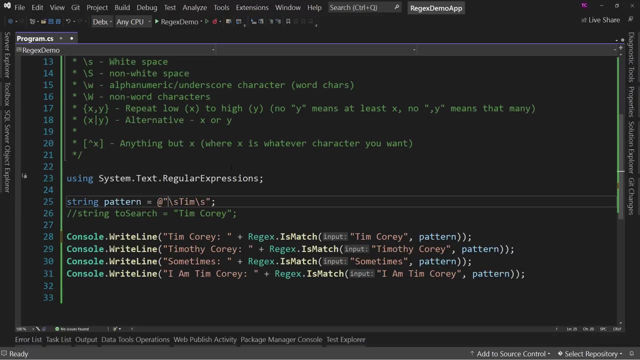 But what if Tim is at the beginning? Well, we've got the option of this range right here, but we also have this alternative. Okay, So X or Y? well, we could say, let's put this in parentheses, So S or the start. 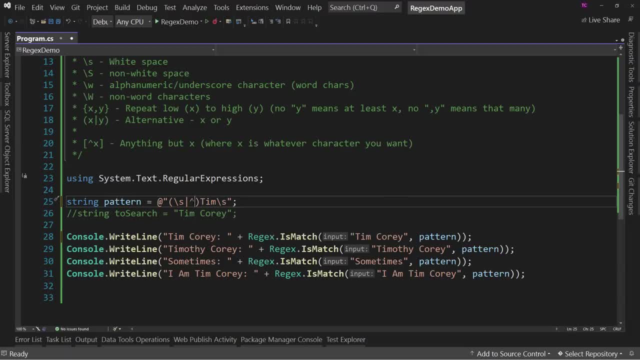 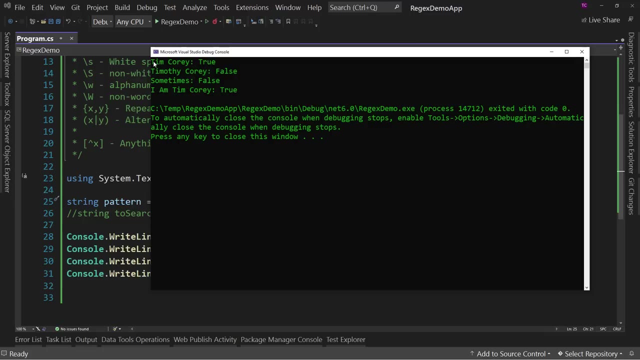 So S or the start of the string, or that's the, or right there or a space. let's run this again. And Tim, I took the space out. Tim Corey is true, So it found it at the very beginning, So now we're finding Tim in more places there. 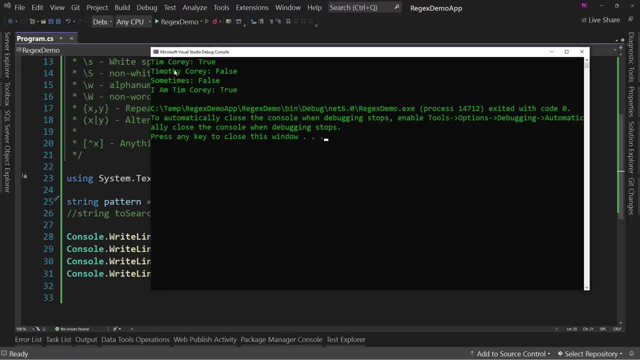 It's more accurate to what it might be in a text file, where we might find that Tim is the first word. Okay, So Tim is the first word in a sentence. you know, Tim went to the mall. Well then, Tim is the beginning of that sentence. 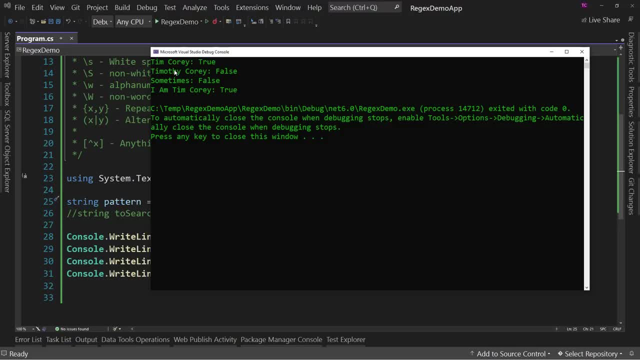 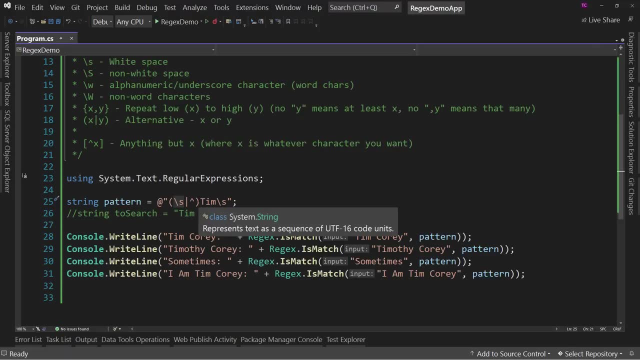 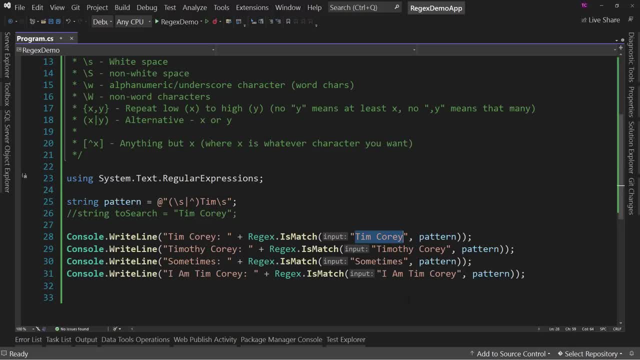 Okay, Okay, Okay, Okay. So let's we know that this works. We know that this works, but let's say sometimes Tim. Okay, Let's say always Tim, because that way there's not Tim in the name to be confused by. 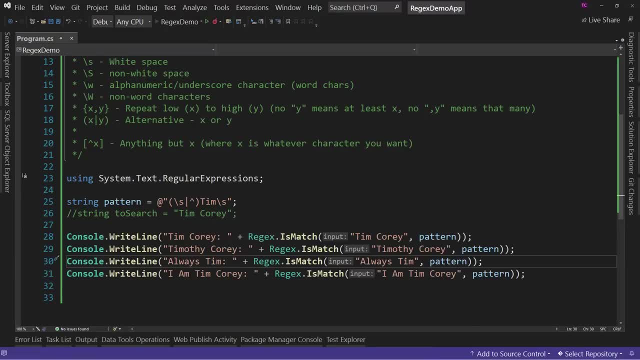 Okay, So always Tim where Tim is at the end. And if we run this, always Tim is false because there's no space after tim. so what do we do? well, we're going to do that grouping there where we say: alternative, so, or? 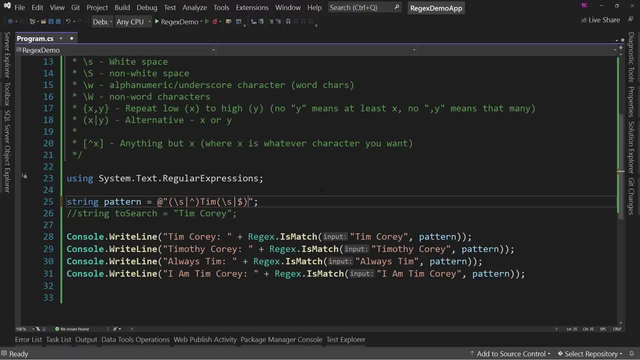 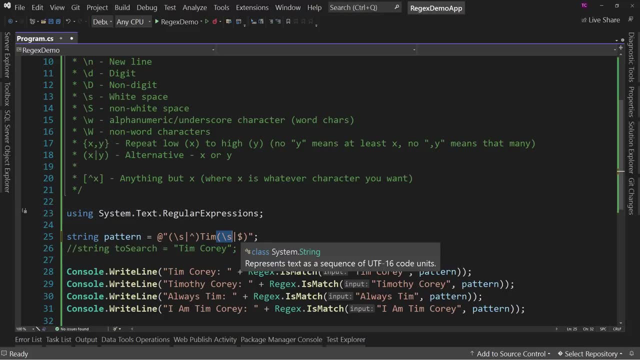 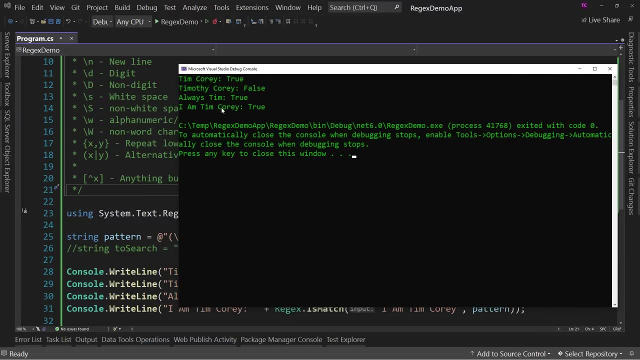 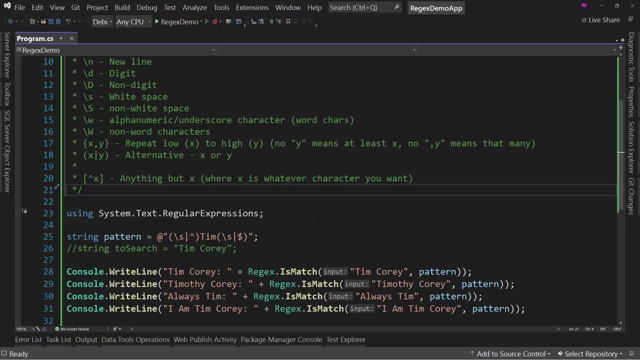 and what's our end character? a dollar sign, how we know right up here, ends with: so either there's a space afterwards or it ends with tim. we run this and we see always: tim is now true. now, i do want to point out at this point that there are other ways of. 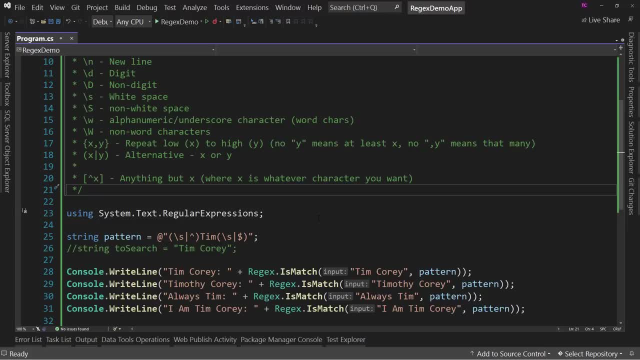 doing these things. this is regular. expressions are like programming in general, there's more than one way to attack a problem and i would encourage you to try out the different ways to see if there's any efficiencies in one versus the other. but just because you can do it in, 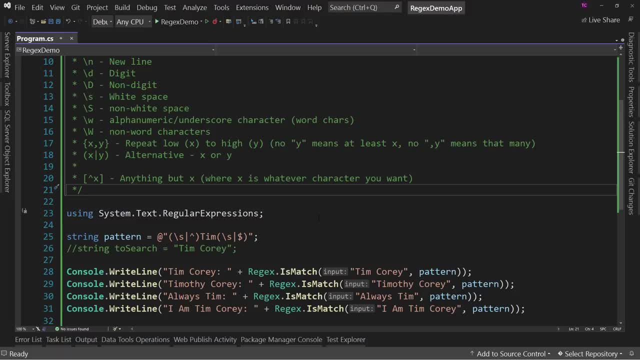 multiple ways doesn't mean that your way is wrong, it just means it's different. and, like with programming, different doesn't mean bad, it means it's different. okay, so with that out of the way, because you may have come across this in a different way or had a different thought on how. 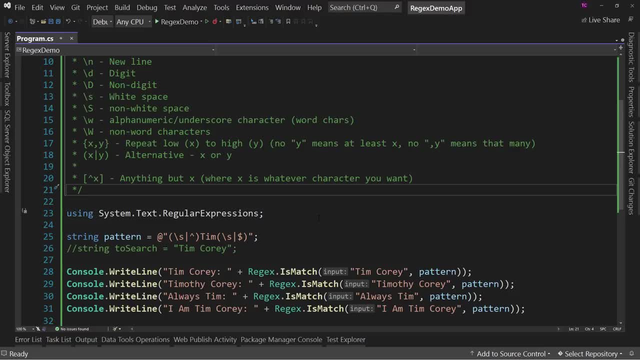 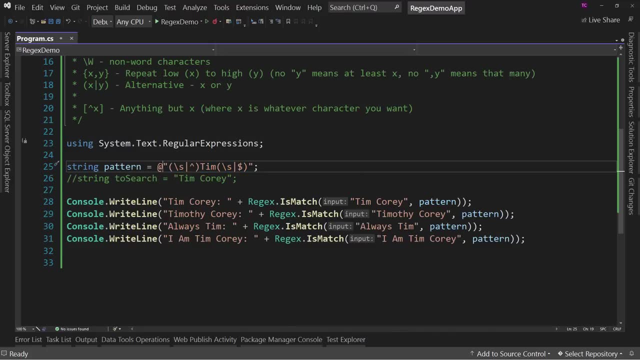 to do this, and that's fine. let's talk about this pattern for a minute. do you notice how complicated it looks? it's got lots of special characters, okay. so at the very beginning, we have one, two and then one, two, three and then one, two and then one, two, three. we have what? 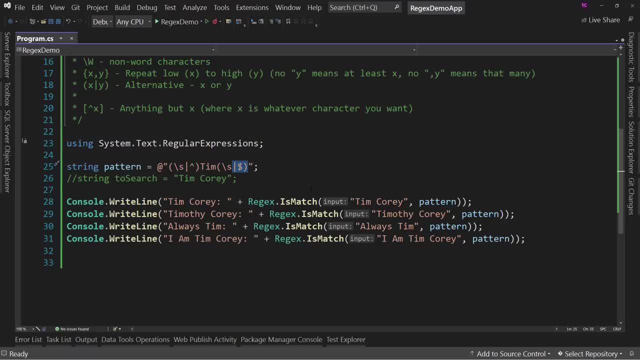 10 special characters with only four we call regular alpha characters, that's- or, i'm sorry, five alpha characters. that looks complicated, but if we started breaking it down and started looking at what it's actually doing, it wasn't complicated, it was just we had to put in all the different 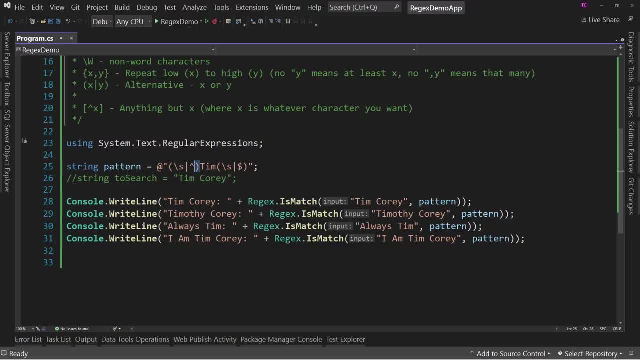 possibilities. so if we start with the very, very simple stuff- just tim, and we start adding a little bit at a time, like, oh, a space before tim, well, a space, or the start, and at the end, oh, a space after tim, or a space or the end, and you start building this up, that's when you get the more complicated statements. 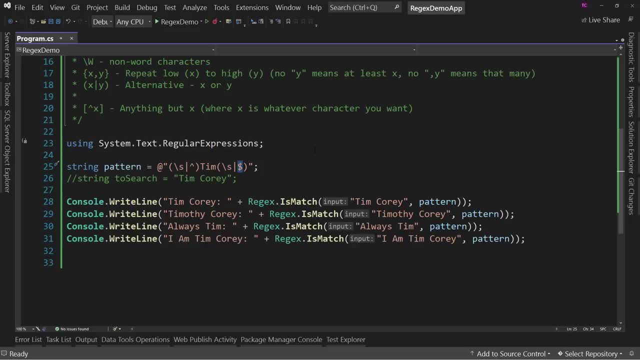 but when you actually take time to figure out what it's doing, it's not nearly as complicated as it looks now. with that being said, you will see some pretty complex regular expressions. i would encourage you to do that if you're a beginner and you're not familiar with the 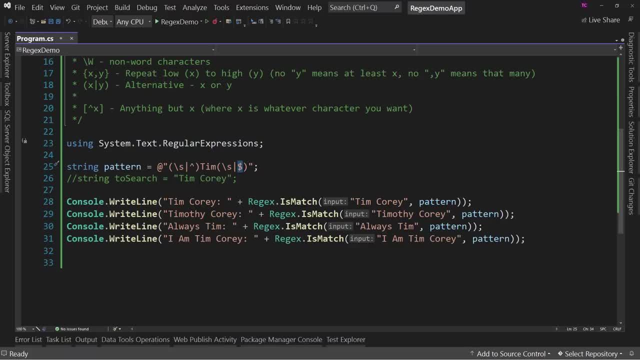 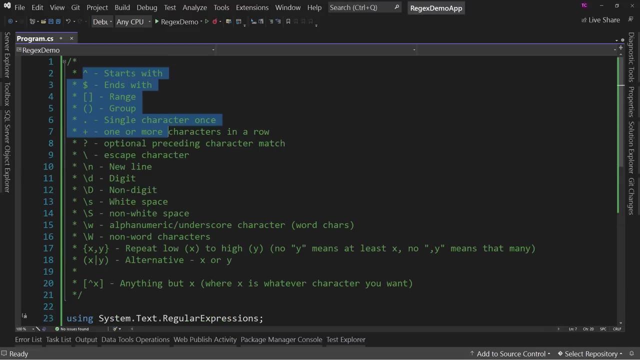 but if you're a beginner and you're not familiar with the, to start off, simple and practice these things. this video is an intro to regular expressions. it's not going to be a comprehensive look at everything you do regular expressions and training you deeply in all of it, but i would encourage you back to here, look at these and start. 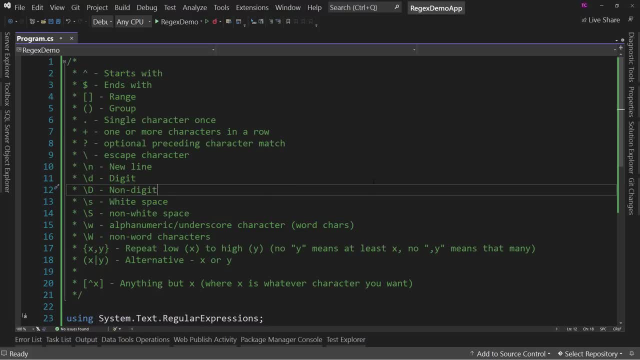 practicing. one of the things i tell people a lot is that the only way to really understand something is to practice it. if you just watch what i do and go, yep, that looks great, i got it. and then try and do it and doesn't work, then you get frustrated. i would encourage you to try this out and practice. 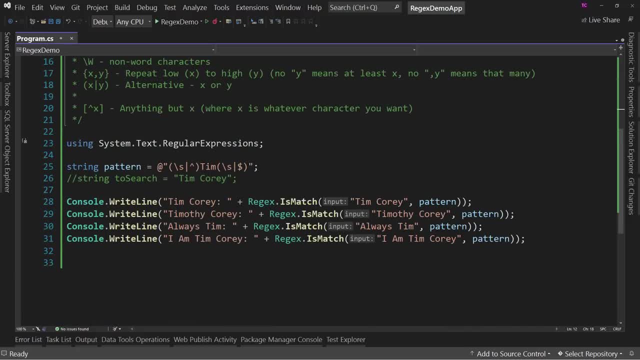 it a few times and start simple. don't start with the complex, start with simple. okay, now let's talk next about this. okay, so we've been using what's called the static version of regular expressions. the static version of regular expressions is a static method. we can call like is match. 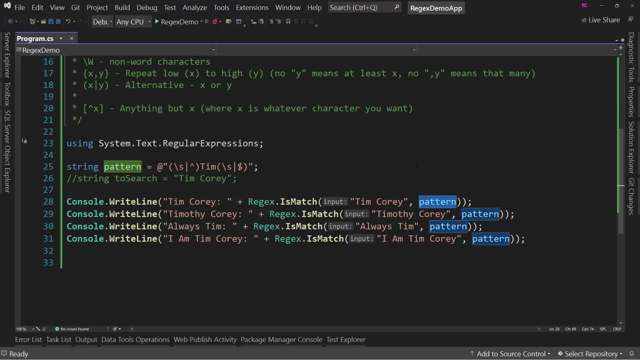 and this passes in the pattern. this pattern is not pre-compiled. so what does pre-compiled mean? well, in regular expressions, c-sharp will turn this into a pattern, a high-level pattern, that it knows about, but it's not in the intermediate language that c-sharp gets compiled down into. 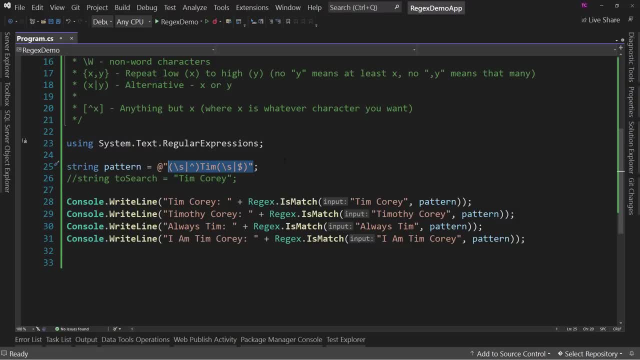 and so when we go to run this, it has to turn this into intermediate language first, and then it runs it. we can pre-compile this, which means that we compile it once and then it's already done, so that it's faster for all of these runs. that's the theory. okay, let's talk about practice. 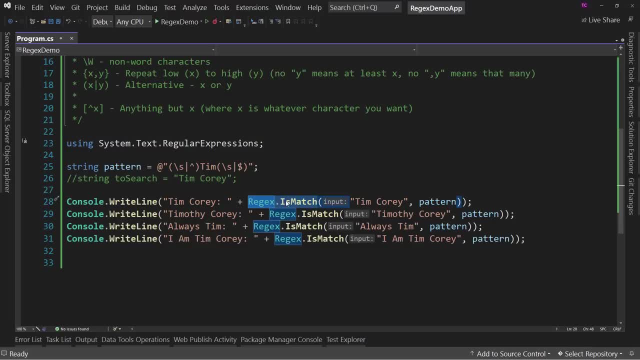 first of all, if you're using the static version- which is what we're doing right here, where it's we just we don't have to instantiate a class- then when you put a pattern in, it's going to compile that and run it, but then when you use it again, it's going to remember, it's going to. 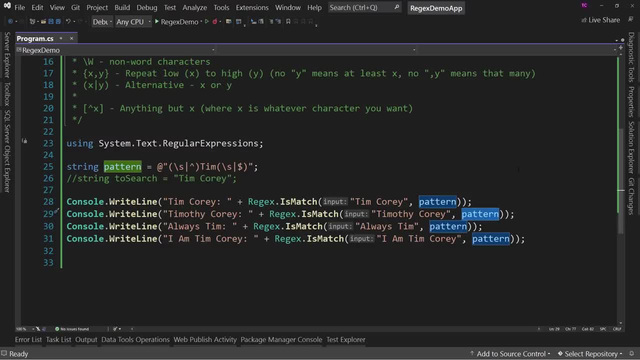 cache that compiled plan and use it over again for up to 15 plans. so as long as you don't have 15 different patterns that you're using or 16 different patterns that you're using, usually fine to reuse without pre-compiling. so that's the idea of the static version of regular expressions. 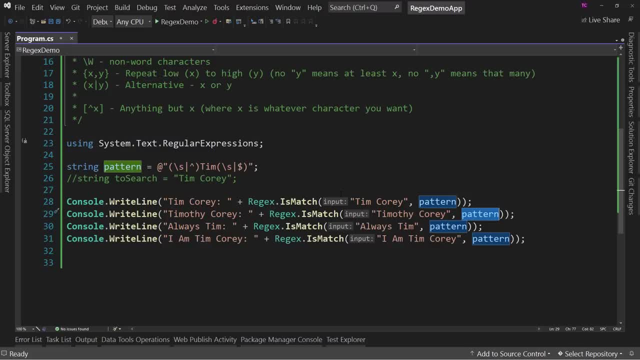 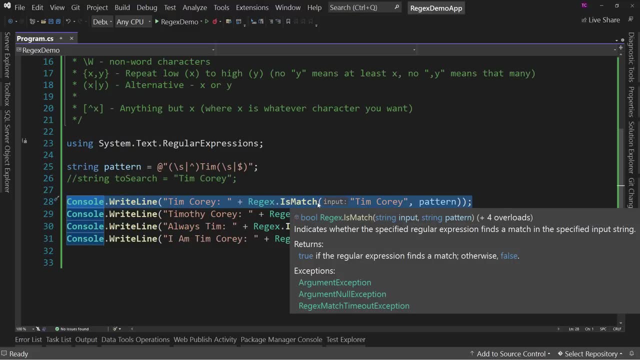 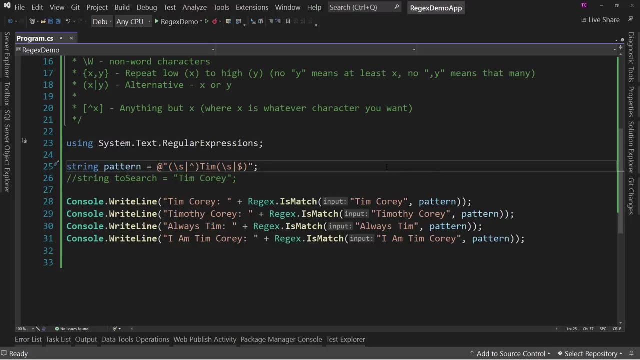 pre-compiling. now the the cost of that compilation happens here the first time you use it. when you're using the static version, you can pre-compile it at the very beginning of your application and then the cost goes there instead. but i want to point out, some people look at regular 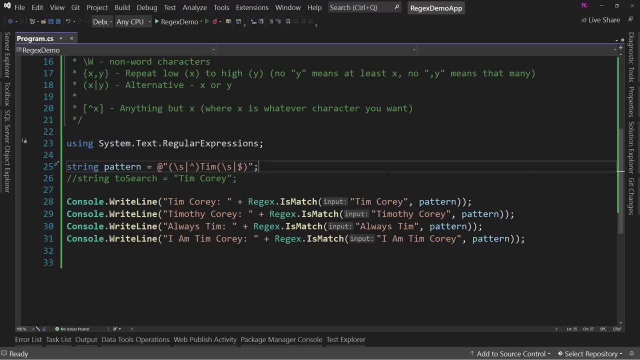 expressions and say, oh my goodness, they're so inefficient, you should never use them and i strongly recommend that you pre-compile them if you're using a static version of regular expressions. disagree with that? in fact, i would like you to test it. so let's do this. let's um, let's run this. 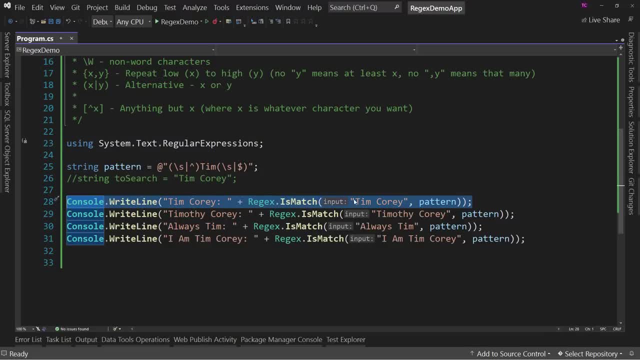 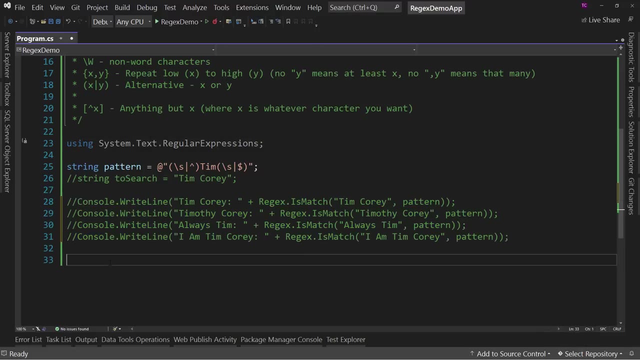 now, this is the, the pre-compiled version. once you run it once, but let's, let's run this um, this expression. what you do is match and return it. true, we're gonna ignore it. okay, so we're gonna. we're gonna copy us or comment this out and i'm gonna say four: 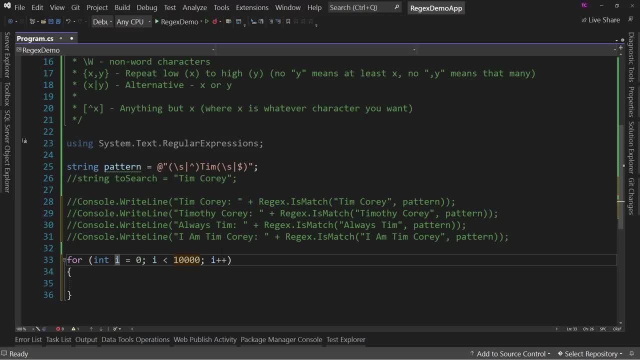 let's do. let's do a hundred thousand. so i'll loop through and run this method 100 000 times. now, is that a lot? yes, that's a very. that's a. that's a lot. okay, so we're gonna run this regular expression match a hundred thousand times. now, what we're gonna do is we're gonna. 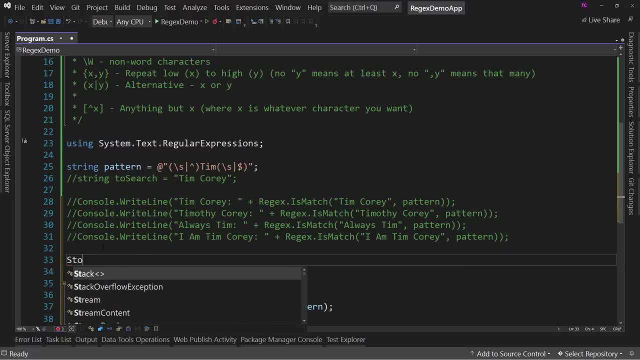 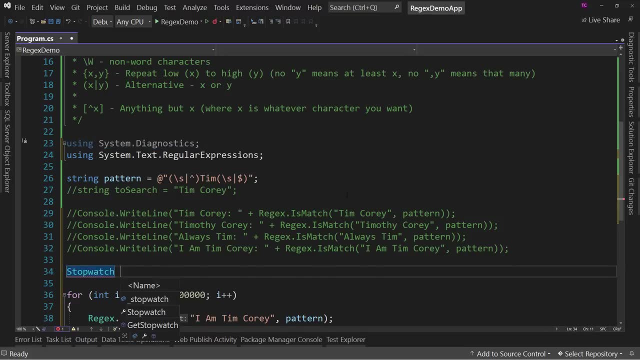 create a stopwatch. so we're gonna say stopwatch and that adds, by the way, the using for systemdiagnostics. we'll call it uh. stopwatch equals uh new, and we'll say at the very beginning here: stopwatch dot start. and then, after this is done, stopwatch dot stop. 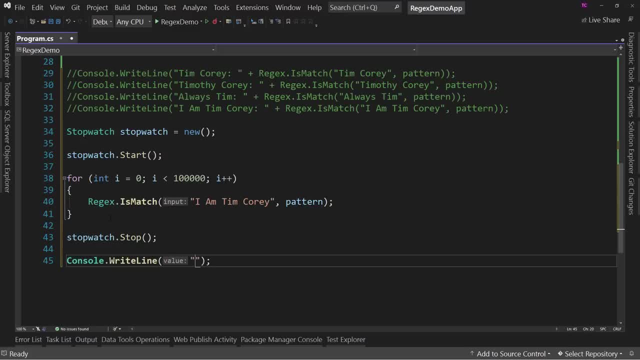 and then we'll print out the time elapsed in milliseconds. and then let's make this a string interpolation. so put the dollar sign in front and we'll say: stopwatch dot elapsed milliseconds: okay. the total elapsed time in milliseconds: okay. now again, this is not seconds, it's milliseconds. we need a thousand milliseconds. 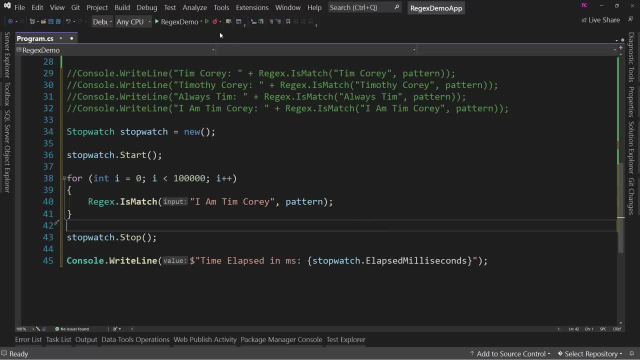 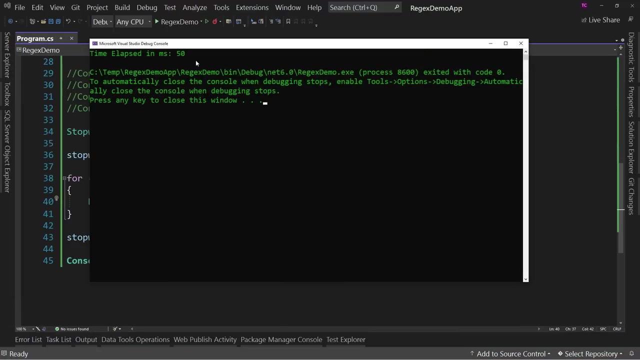 thousand milliseconds in order to equal one second. so we're gonna run this 100 000 times now. yes, the first time it runs it will be compiled. after that it'll use that cached version. let's run this. it's done. we've run this in 50 milliseconds, 100 000 times 50 milliseconds now. 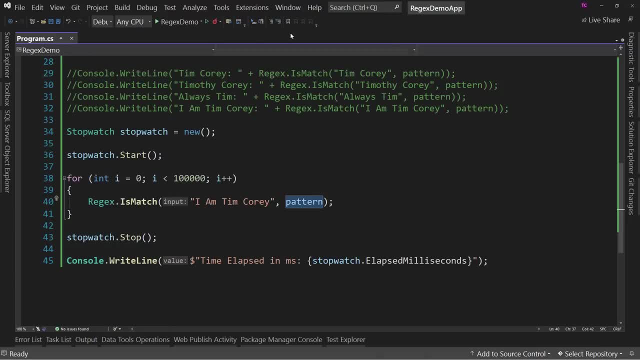 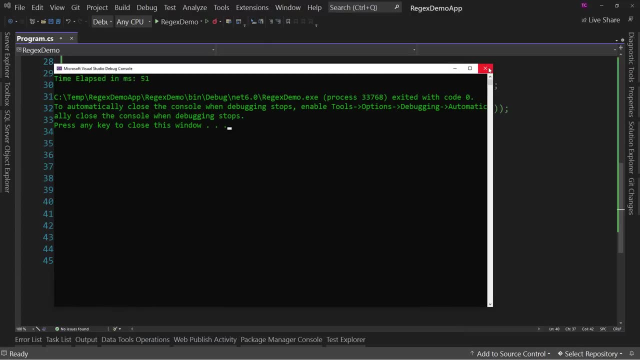 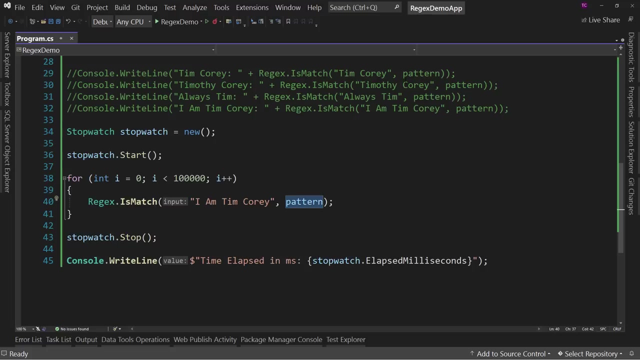 let's run again. just want to show you something: 50.. let's run it again 51.. let's run it again 51.. your computer might be different because you might have a different cpu, whatever, but it's pretty consistent around that. but it's so minuscule as far as time goes. 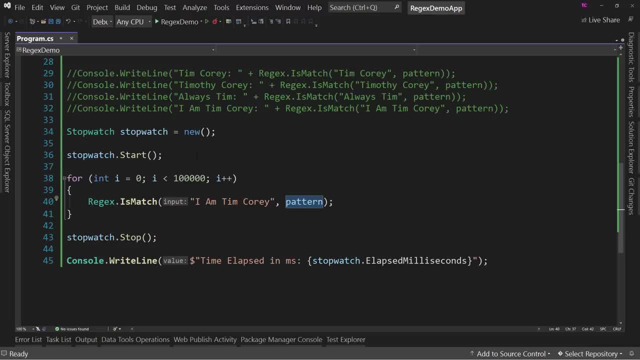 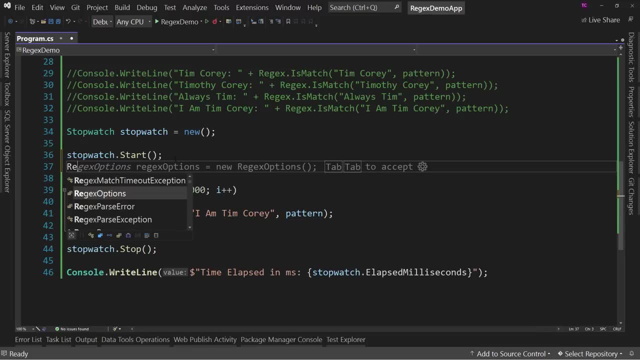 that a little bit of variation is fine. now let's change this to a a not compiled statement. so we're going to say: uh regex, uh test equals new regex with a pattern. all right, this is instantiated version of a regular expression. now, when you use an instantiated 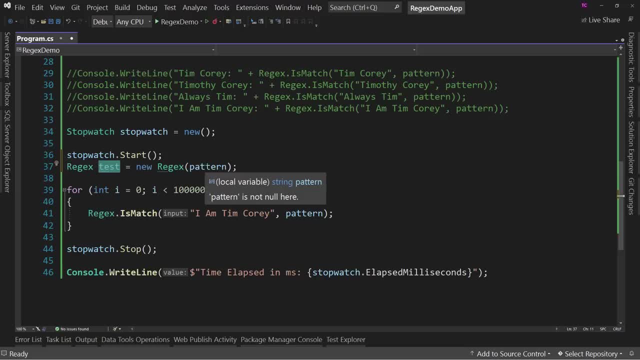 version. you can pre-compile it, but if you don't, it will never be compiled or cached. i'm sorry, it'll never be cached for the next time. it'll always be compiled every time. so let's take this out. this is about 50 milliseconds, right. 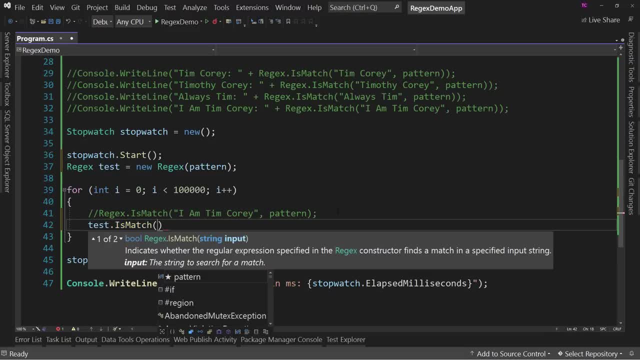 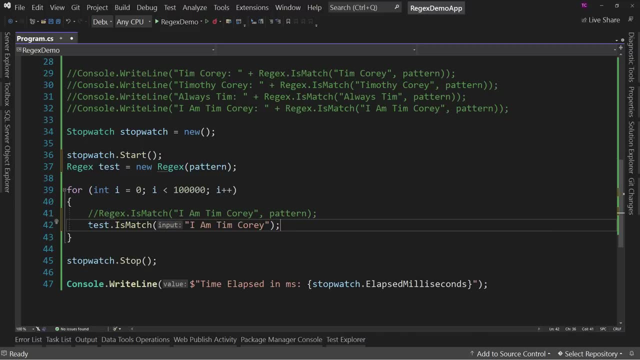 we're going to say test dot is match, for i am tim corey, it's the same thing, it's just using the instance which passes in the pattern ahead of time. but again, this is the not compiled version yet. so let's, and we're putting this inside the start. so 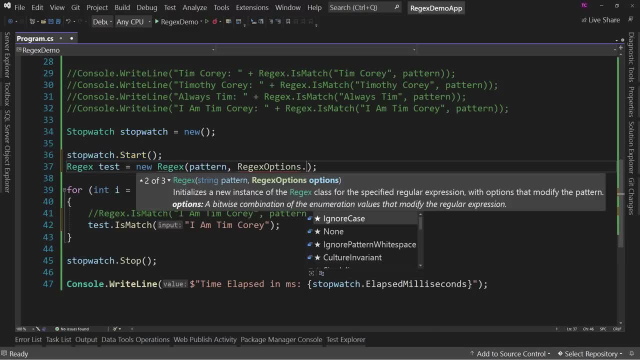 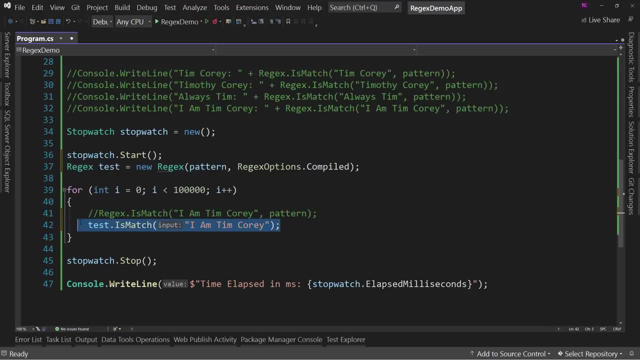 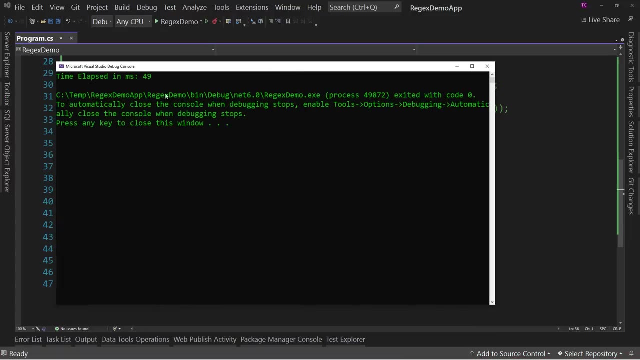 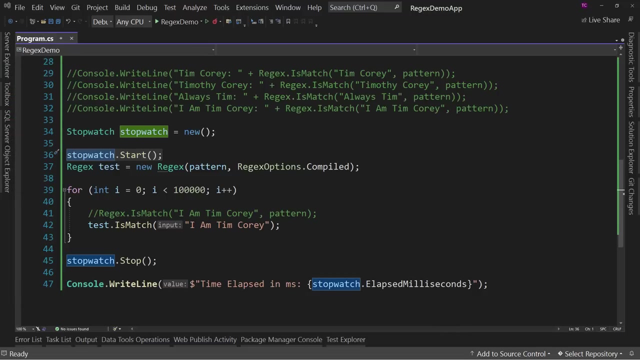 even if we compile, let's compile first. dot compiled. it says we'll compile it once and then reuse it over and over again. but again, we're testing it inside of the stopwatchstart: 49. okay, 49 milliseconds. let's run it again 50.. 47. 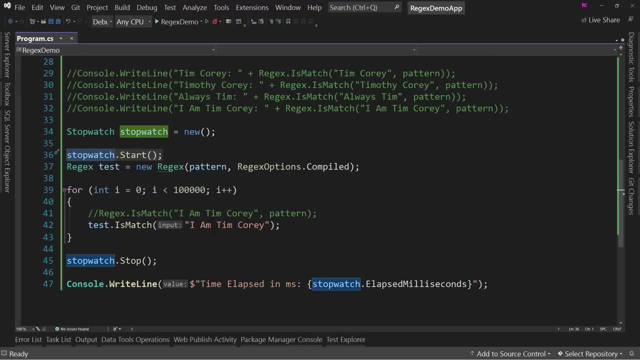 49 about the same. i mean, the variance is so little it's not really a variance, because the fact that you know anything can affect this. now let's not compile it, which means it's going to compile itself every single time. 41, 42, 43. 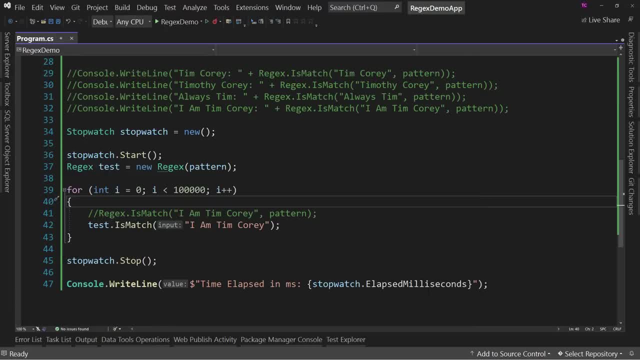 41, it's actually a little faster. so when people start to freak out and say, oh my goodness, this is a thing you should never do. it's so dangerous, it's so expensive, listen, regular expressions can be expensive. don't. don't hear me say they're not. however, 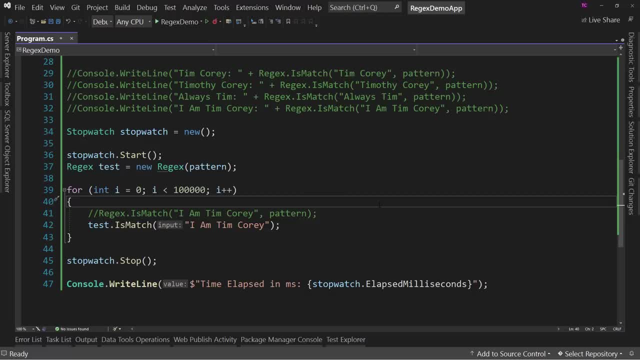 when we say expensive, we don't mean never use them. never use them. what it means is be smart about it. if you have a loop with a million records you're looping through and then you're running three or four different regular expressions on them, yes, that's gonna be slow, but it might be necessary. the other part is: can you do this without? 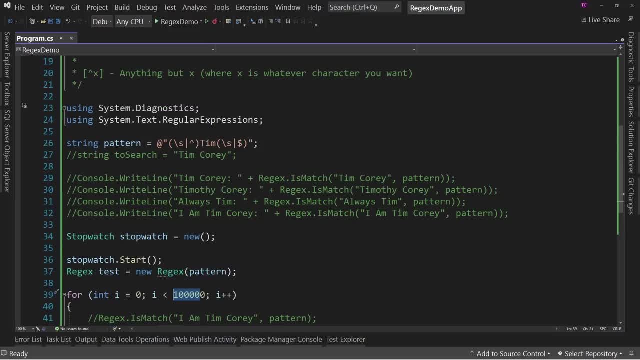 a regular expression. so in these i could have said: contains, you know so, does this contain tim? i could have done that. now this not so much. this is harder to do. i could have said: starts with tim, or ends with tim, or contains tim. i could do that, but that becomes like three different statements. 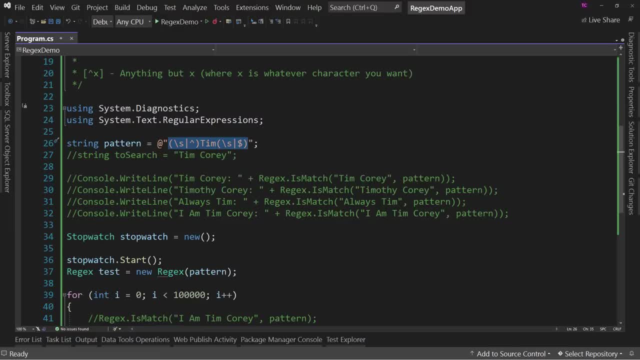 to run, which is where a regular expression starts to shine. so just saying, look for tim. we could do this another way. but if you're saying, hey, i want you to find this pattern of things, that's probably to be a regular expression and it's okay to run. it. just look for any time you're. 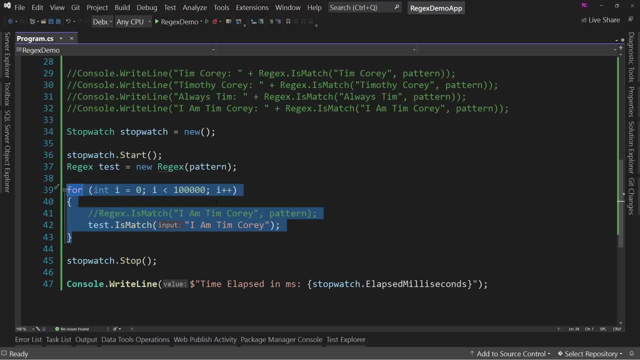 running up millions of times, then you need to benchmark and figure out if there's a different way. but if you're running this ten, 100, 500 times, even you're not going to see a performance hit at all. but again, you should test in your scenario. you should know what um where the performance. 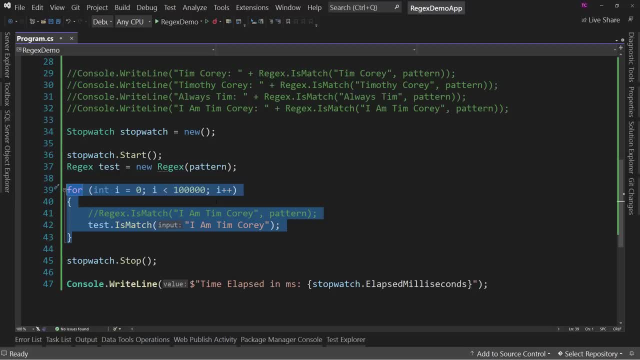 bottlenecks are in your application, but performance bottlenecks are something you should try to get to to wear them right. you shouldn't run a perf iki in your Ahhh, muy bien know, just to run them on your app. bottlenecks are something you should find probably near the end of your project, rather than trying 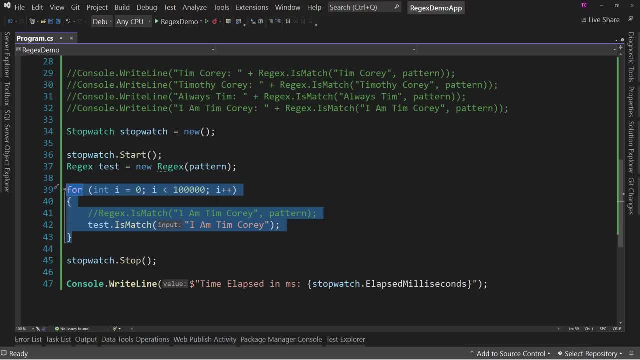 to pre-do all of your efficiencies. If you say you know what, we're not going to use regular expressions because they're slow, That's a bad take. This is a tool that is available. It is the best tool for the job in a lot of circumstances. So be careful with some of the 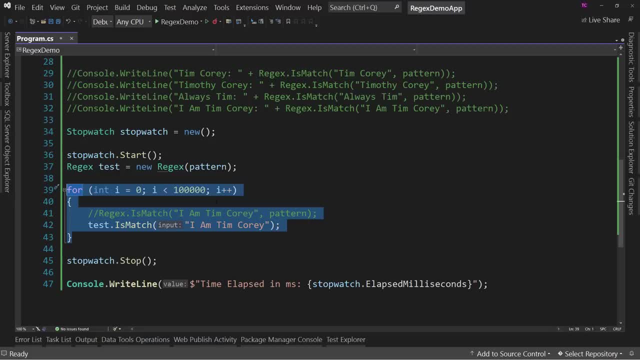 rhetoric around regular expressions because, quite frankly, it's not helpful to what we're doing And it actually hurts you as a developer to not have this tool in your toolbox. So I just want to point that out that they're not nearly as inefficient as you thought they were, especially 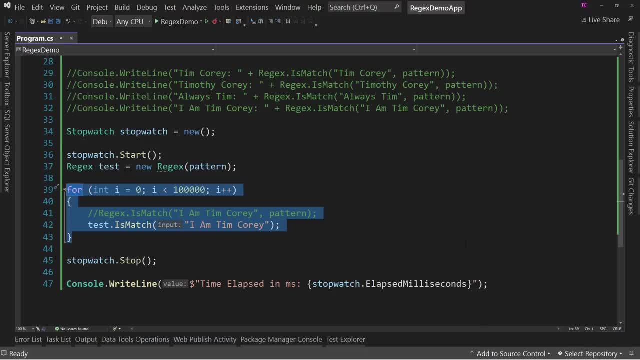 not in newer versions of NET. Now, if you go to NET framework they might be slower. but in NET 6, what I'm doing right here- super efficient And, again, always test. You can use a stopwatch, Just try it out. There's other ways of testing performance. 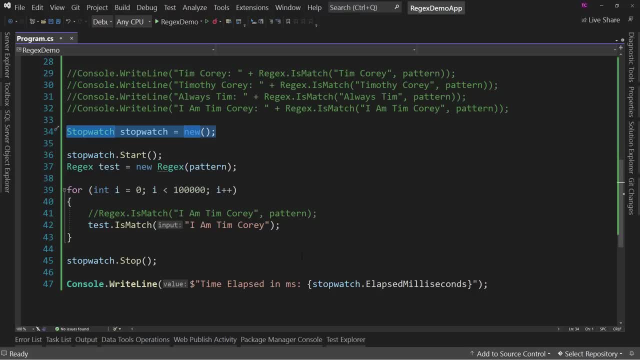 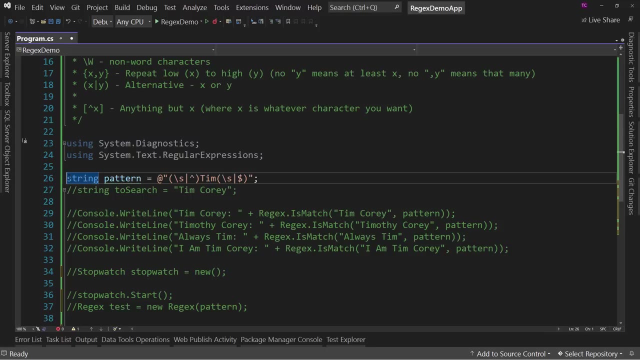 but this is a quick way, in a little console application, to test just that one line to see how efficient it is. Okay, let's keep going, And what we're going to do is we're going to take on a more complex scenario. Now, let's do this, Let's move this up to the very top. 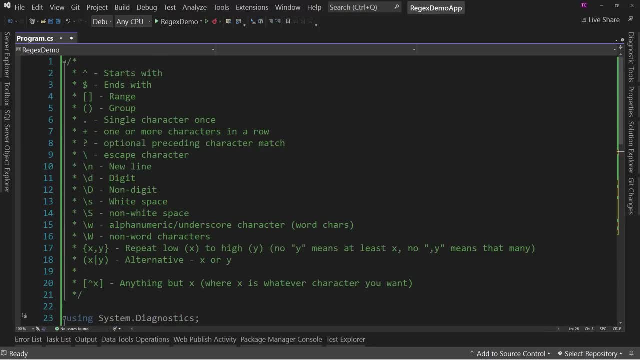 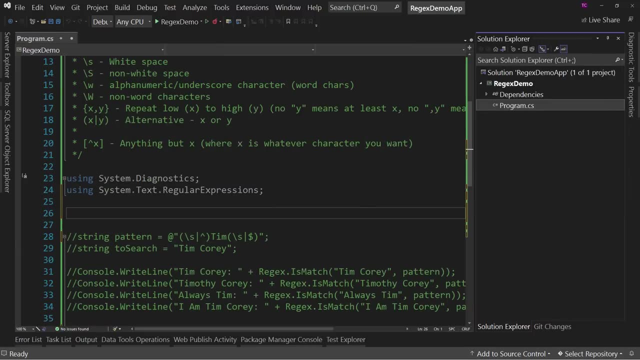 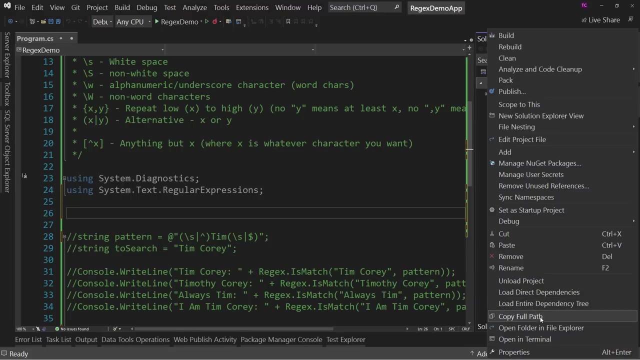 because I want to get close to this. We're going to use this quite a bit And what we're going to do is: let's bring my Solution Explorer here. I'm going to copy a text file. I'm just going to paste it in there. I cannot. Well, no problem, I'm going to open folder. 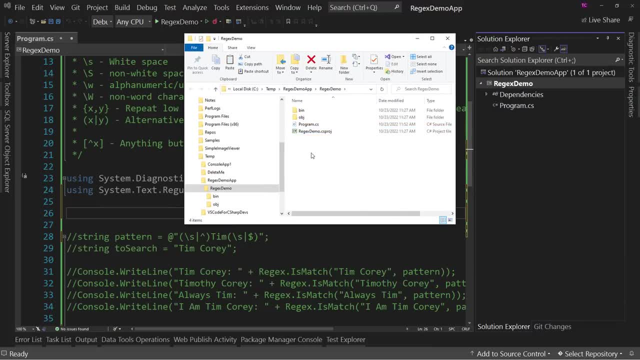 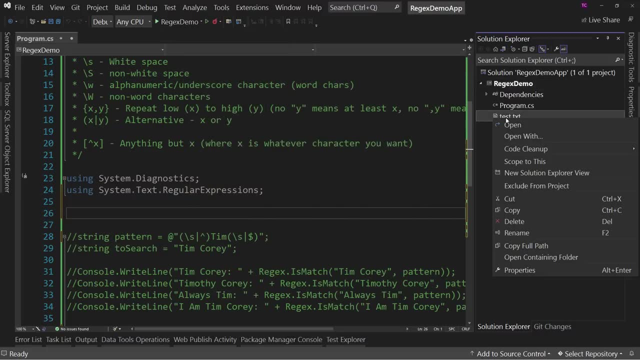 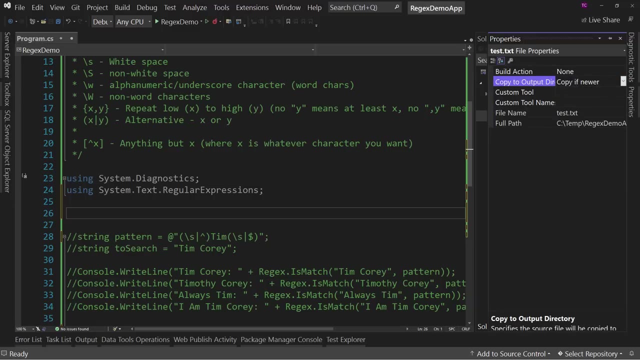 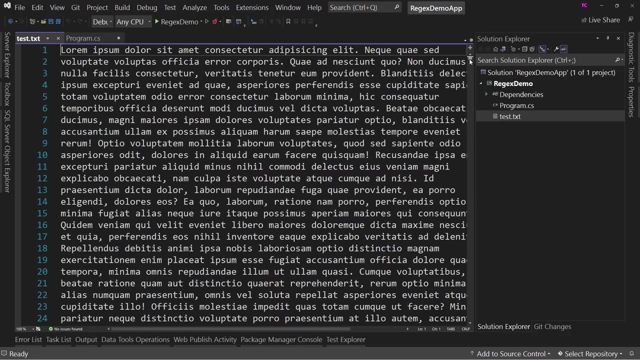 in File Explorer and I'm going to paste into it a text file, And it's right here: testtxt. Now let's go to the properties of this and say yes, copy to the output directory. And what is this? It's a text file, And if we look it's a big text file. 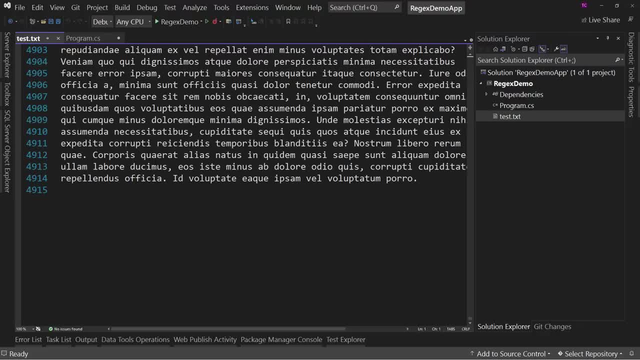 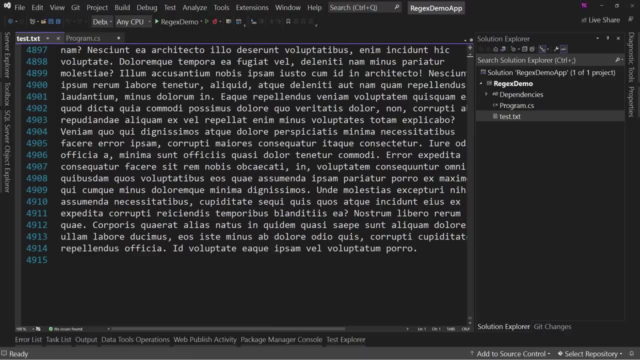 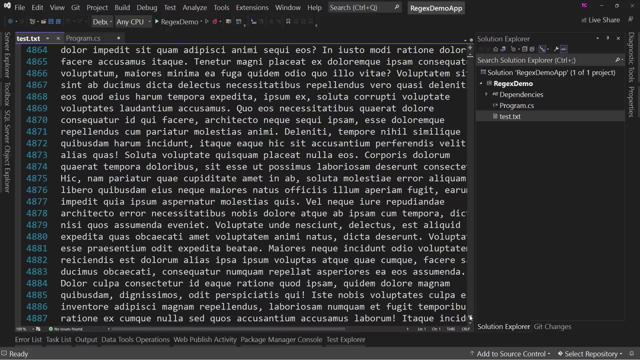 It's just almost not quite. it's almost a thousand lines, I'm sorry, 5,000 lines of text And it scrolls off to the right. I think it's about 80 characters wide or something like that. This is Lorem Ipsum text, So I went into. I didn't use an online text, but I did use an online text. 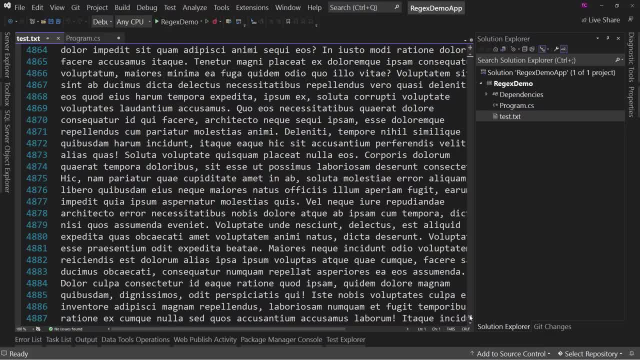 I went to VS Code and created an HTML document and said Lorem, and I think it was- oh goodness, I think it was 50,000. I asked for So 50,000 words in Lorem Ipsum text and I formatted it. 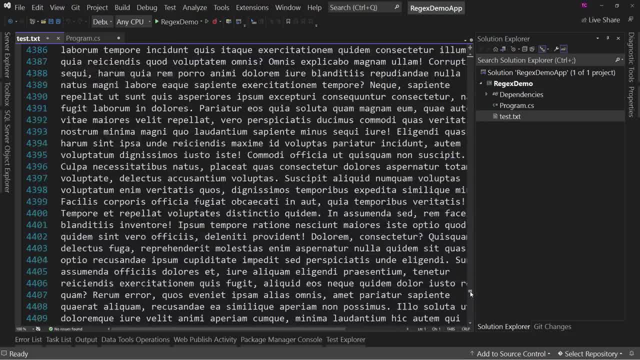 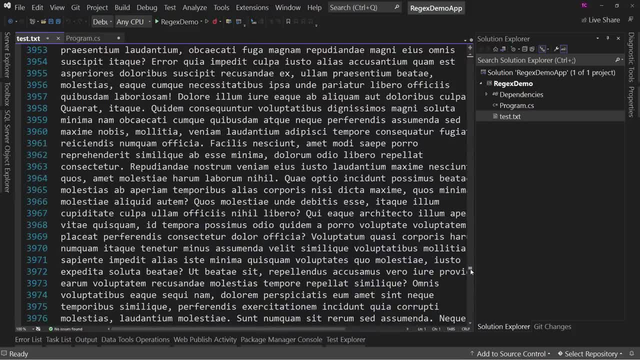 and saved it. But then if we look in here, I'm sure you'll see it just by scrolling through right In here, somewhere are six phone numbers. Now I'm going to give you a way to find them without a regular expression. 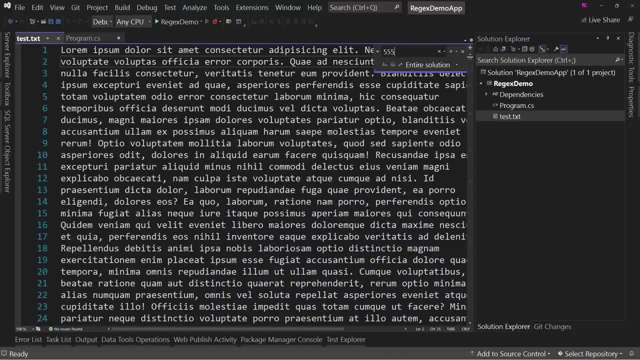 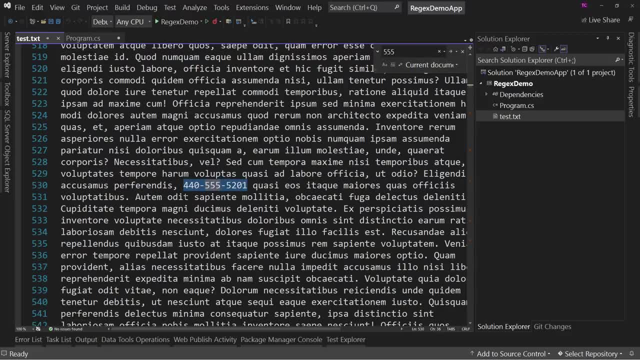 You can know where they are. Do control F and look for 555.. That's in every phone number in here. So the first one is this one. On live 530, there's 440-555-5201.. This is a. I used US format for. 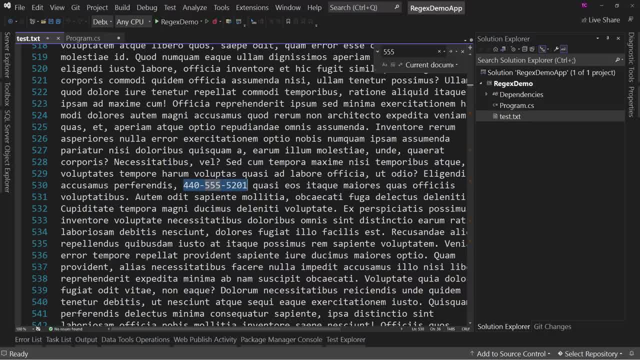 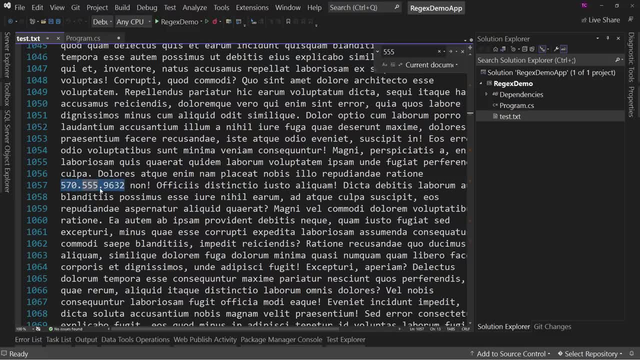 phone number. We're just going to stick with the US format. Okay, But there's one with dashes in between. Let's go to the next one. Well, this one at the beginning of the string, and it uses dots instead of dashes. 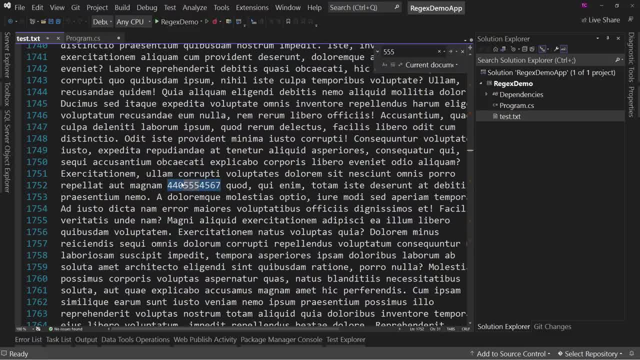 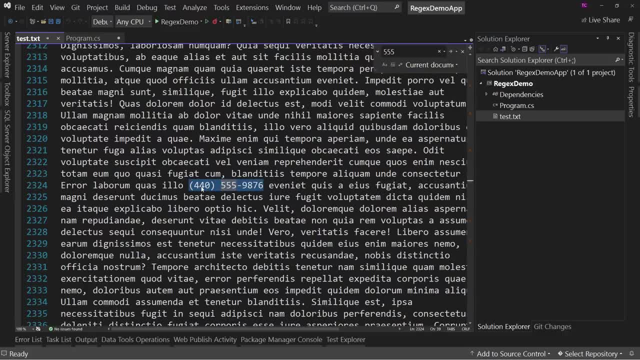 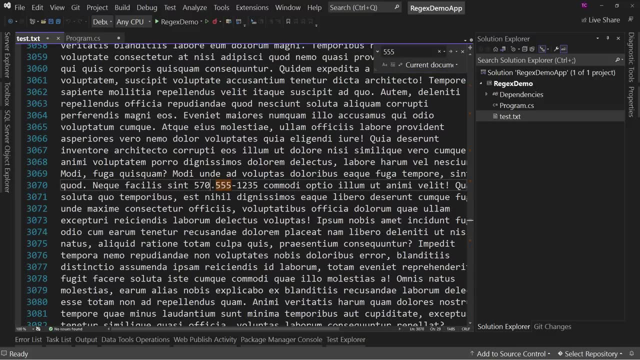 This one. it's a phone number but there's no separators at all. This one has the parentheses around the area code, a space and then a dash here. And then this one kind of has mixed: It has a dot and a dash. 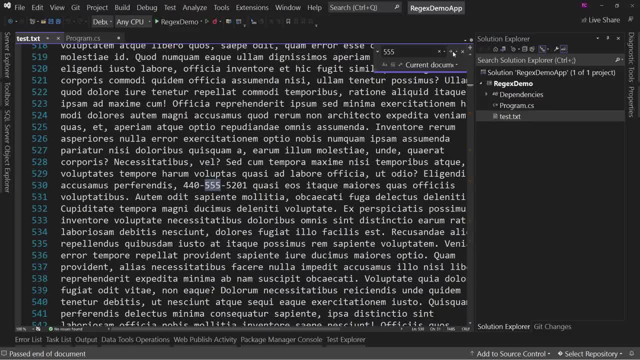 And we have dots down here. I think that's all of them. Yep, Back to the beginning. So that's our options For our phone numbers. Those phone numbers are hard to spot and they're kind of buried in here. The only way we really find them in this mess is if we one looked for 555, which I included in. 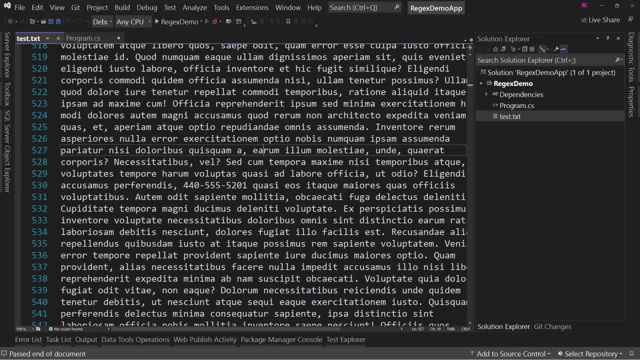 there on purpose or we look for any kind of digits. But what if there's other kinds of things in here that have digits? Well, that's going to create a mess, because there's a phone number in here, possibly, but is it a phone number or is it an ID? 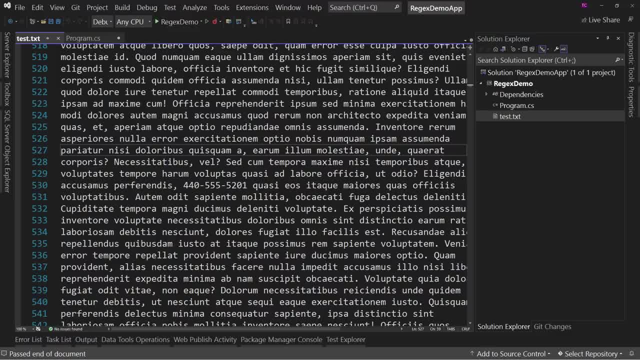 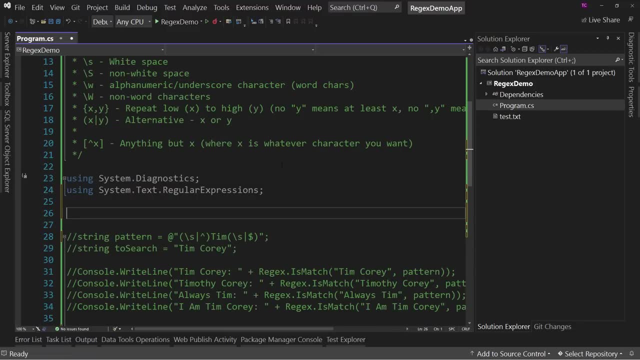 Or is it a zip code, Or is it. and so we want to do is take this text file and use this to really show off how powerful the regular expressions can be. So what we're going to do is we're going to look for those phone numbers in that text file. 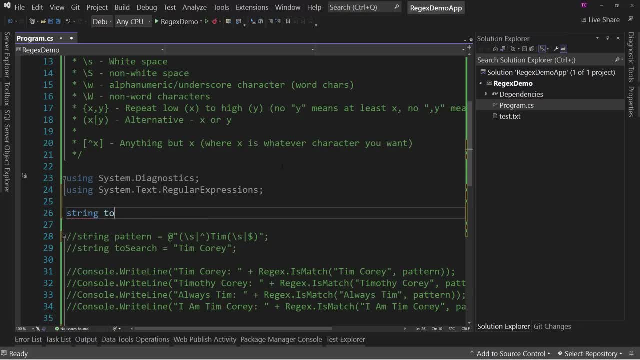 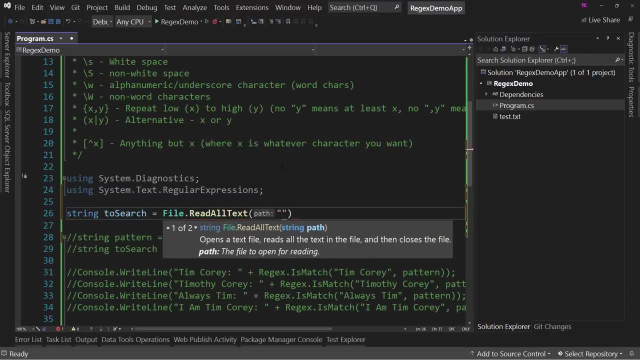 Let's start by looking up the file. So we're going to say string to search equals file. that read all text From testtxt. Now something to point out here. first of all, I'm reusing this variable. It's declared down here, So you cannot just uncomment everything and have everything run. 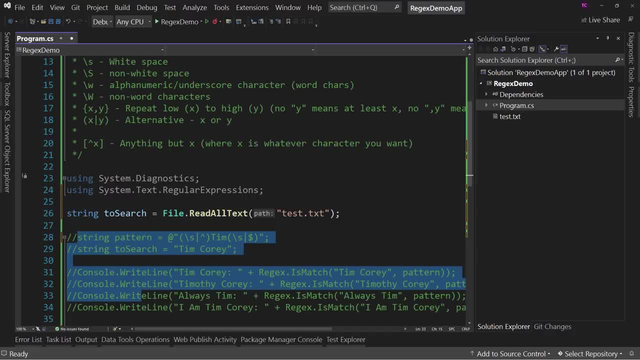 You can comment this out if you want to uncomment this. So I wanted to name it the same because I wanted to be as clear as possible. But then also we're reading all text. Now there's different ways to read a text file in. 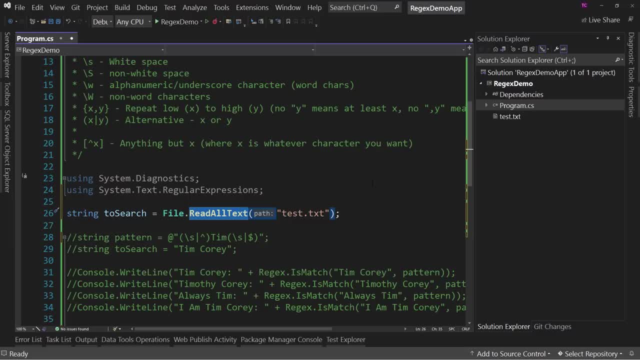 You can read all text, you can read all lines and so on. we're going to read all text, which means that all 5 000 lines, or almost 5 000 lines, of lorem ipsum text is they put into this variable as a string. the whole thing. now, if you had a million rows, that might not be efficient. you might have to stream. 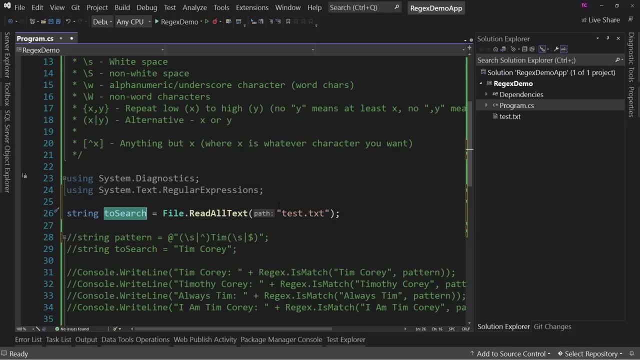 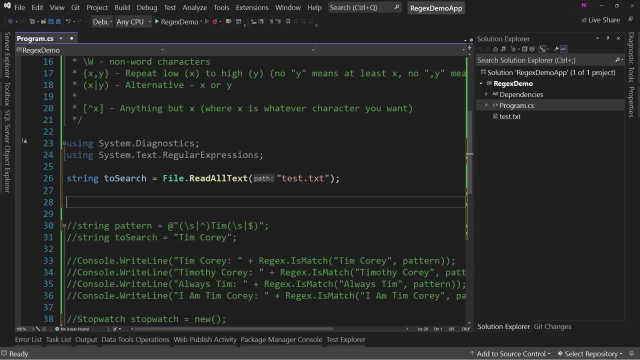 the text file and then run it the real expression multiple times, which you could do, but in our case this works just fine and it's efficient. so we're going to grab this, but i want to make sure that we have everything. so let's do this. um, let's just say: well, let's, let's create our pattern. 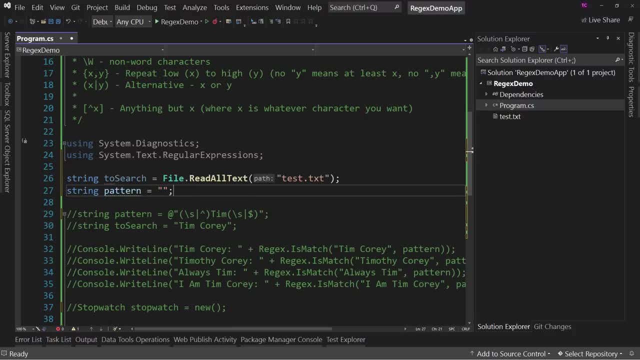 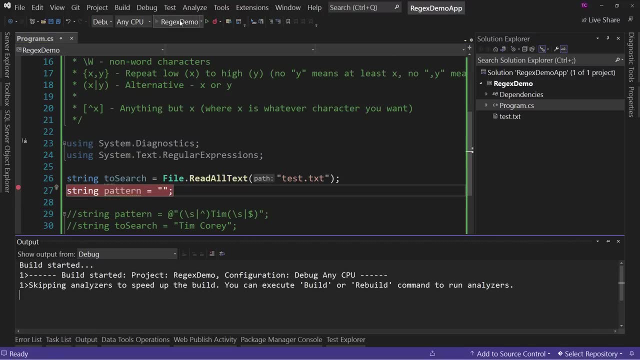 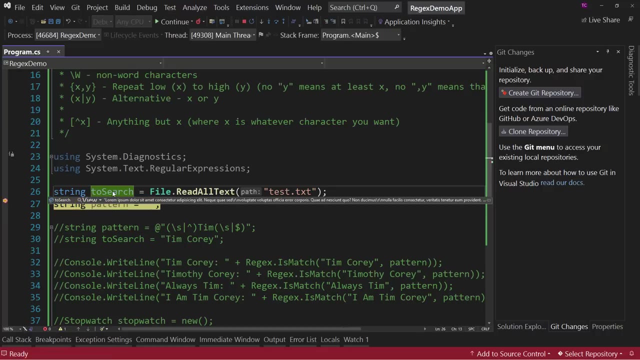 string pattern equals. but then just put a break point here, okay, and we're going to run this just to make sure that to search fills up. that's all we're going to do. breakpoint is hit and to search, if you notice, has a lot of stuff in it, okay. so if we mouse over it and look, it's got a lot. 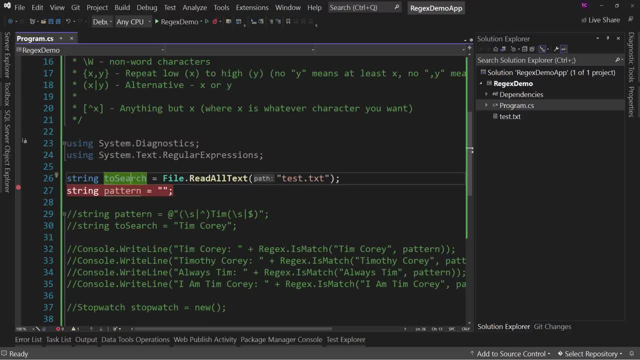 now that means that we in fact did read from our text file which the text file is located, without a path. what does that mean? it's finding it in the same location as our executable. that just means that when you go and download the source code again, you can. 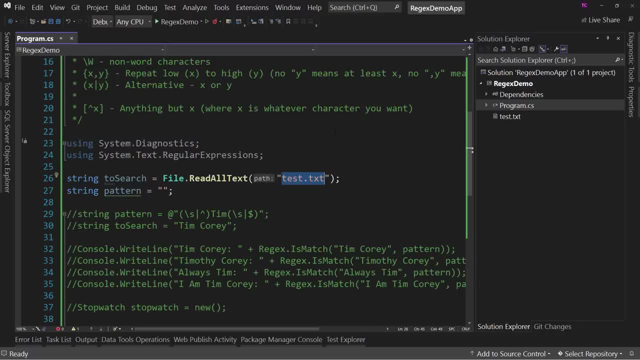 get the source code by using a link in the description. but if you get a source code, then it'll work for you too, because i have it on my machine in different location than yours, but because i put it into the project and said: copy, if newer, it's going to put it in the same. 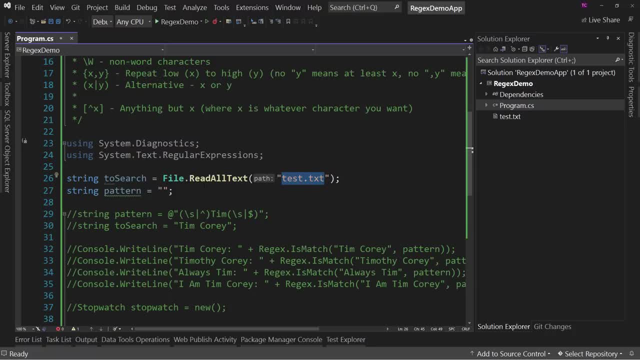 folder as the compiled executable for our application. so now we have the entire file in this variable. now we have a pattern to create. so that's next, and what we're going to do is we're going to try to get all the matches we're going to. 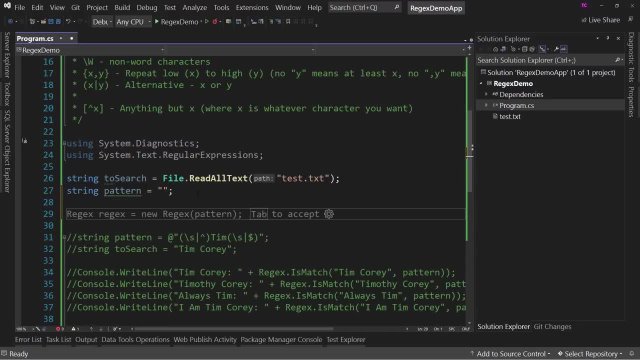 wait on the pattern for a minute and we're going to say match collection, or call it matches equals, and it's actually already telling me what i should probably do, which is regex dot matches. again, it's the static version and we're saying: to search. that's the the place to search, so that's. 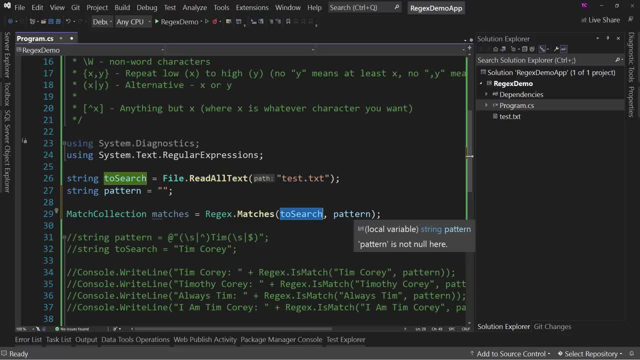 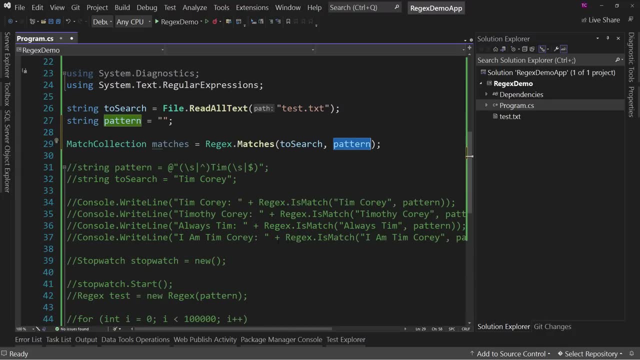 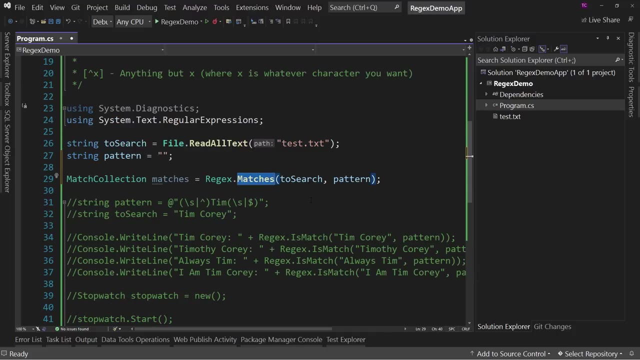 where we're looking for the matches and the pattern to find. is this string right here and so this matches. notice it's not the same as we did down here, which is: is match. is matches said yes, i found a match, but matches says hey, find me all, not just one, but all of the times that this regular 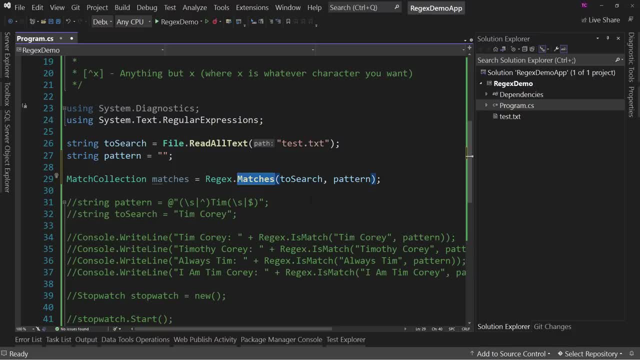 expression matches and what the match was. because, again, we're not going to look for a specific phone number and say is it in that file. instead, we're going to look for a phone number pattern and say what phone numbers do you find there's a difference? so with our matches we have what to 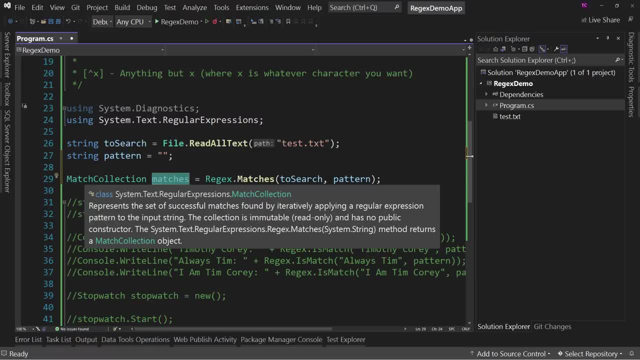 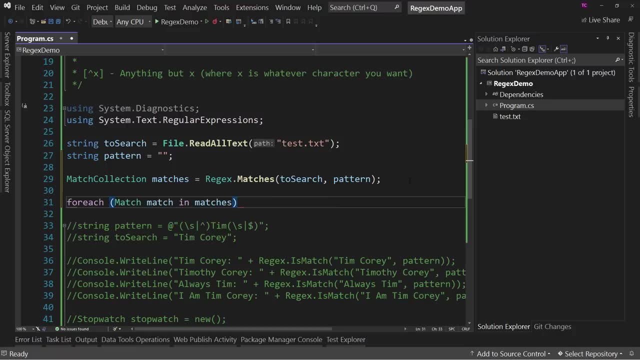 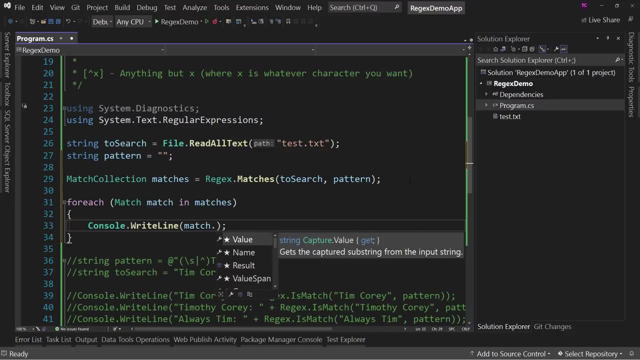 search and the pattern it's going to return a match collection which is a set of matches, and then we can say for each match in matches and we'll say console right line and we can just say match, which is a, you can say matchvalue, like so, and that's just the actual printed out. hey, we found this match. 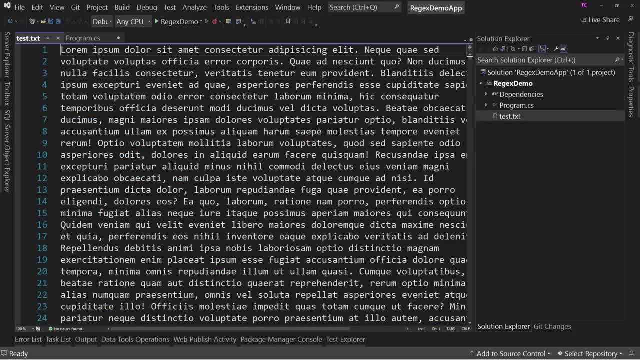 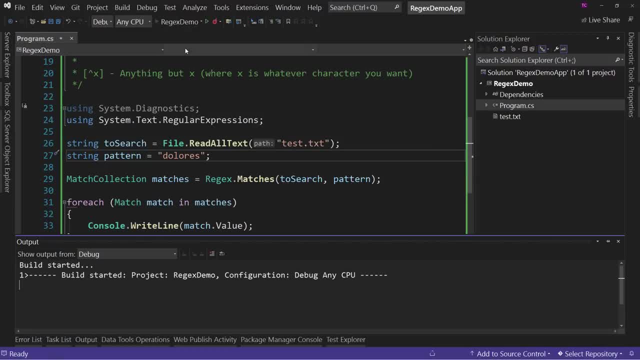 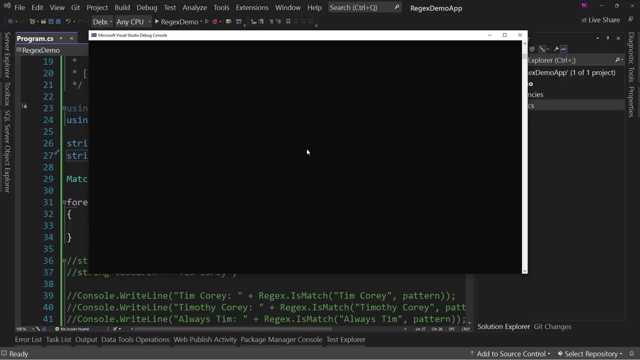 um. so with our text file we could find something like: let's just look for dolores, right, if we do this pattern match and we run this, we'll see it found. delora's a lot. that's because it uses um. it uses that word over and over again when we're doing our lorem ipsum text, we're not looking. for dolores. we're trying to look for a text and we're going to raise the text of the pattern next time. we're going to look for a common text, so we're going to use a cs4 type in our description. but the answer to this is that, dolores, do we know what it is we're looking for? maybe in class or x universe? i'm good to know about this. we're not ignoring six or five time ten. this is a statement. 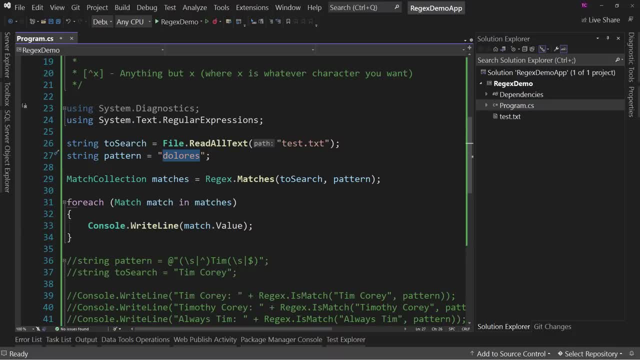 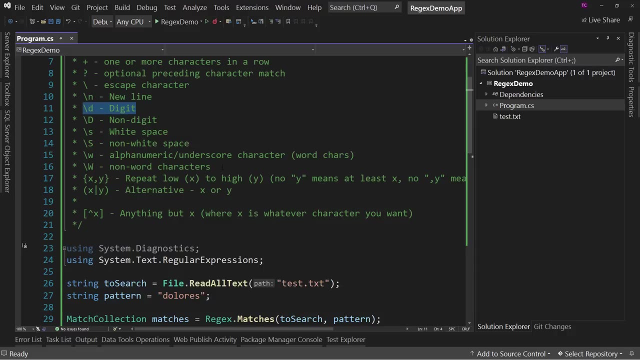 not looking for Dolores, We're looking for a phone number. Well, let's define a phone number. What is it that makes up a phone number? Well, it's going to have digits. Now notice here we have slash D lowercase, which is a digit character. So we're going to want to find. 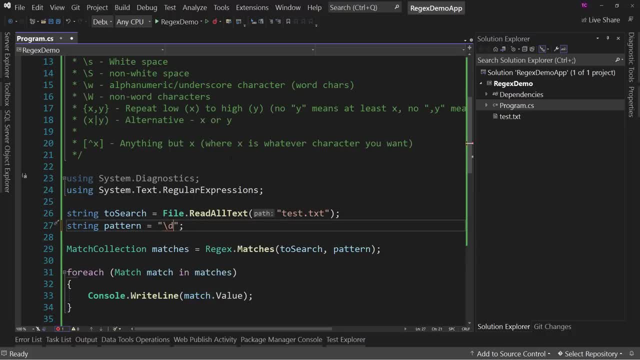 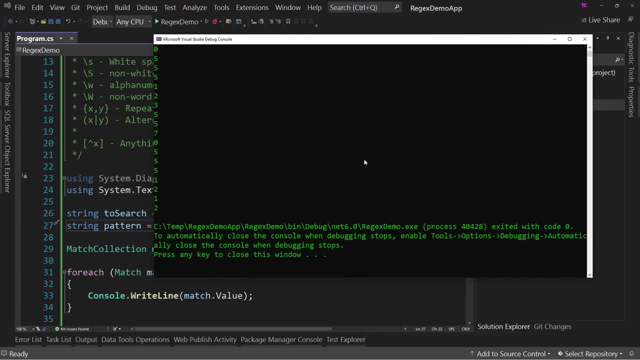 a digit character. Now, if we just said oops, we say that this is a string literal. So if we said this is we just want to find a digit character, it's going to find a lot of them. In fact, if we run this, there's all the digits found, but that's not really a phone number. 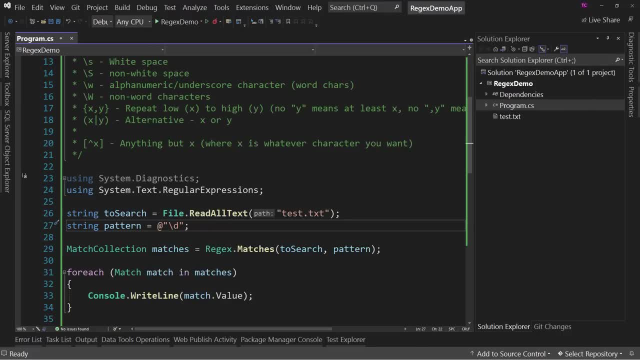 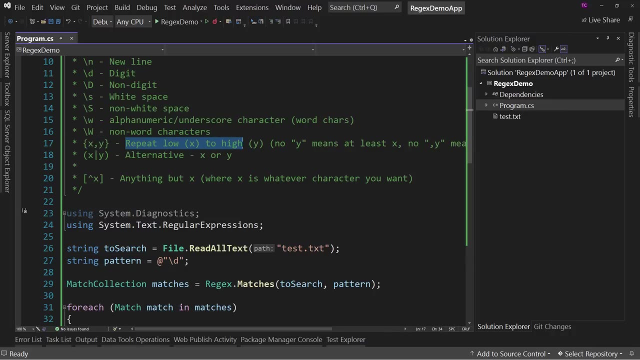 That's just finding. every place we find a number. We want a pattern of numbers, So we want three digits. together is the first section, And we have the ability to use the curly braces to find a repetition. Now this pattern right here says repeat low to high, So one to three of whatever. 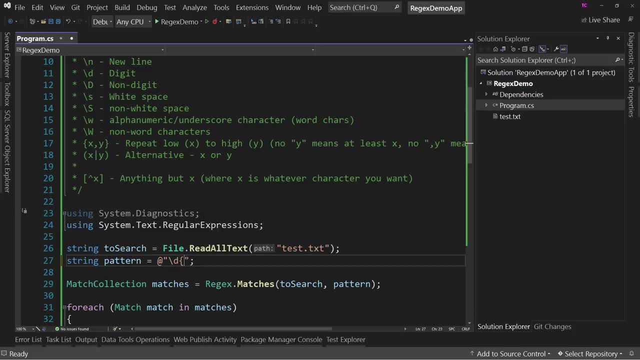 precedes it. So if I were to say, you know, one comma three, this would say one to three digits. but we don't want that. We want three digits. Now, if we don't have the end the Y, that says at least one. 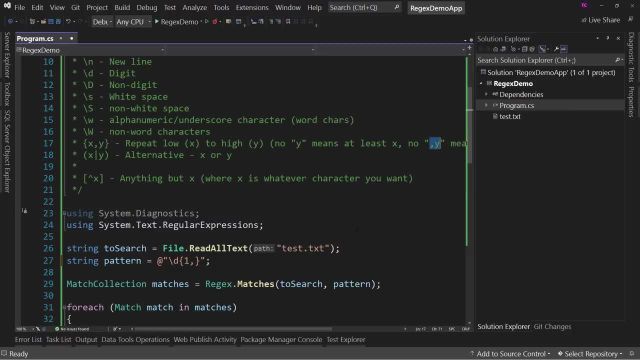 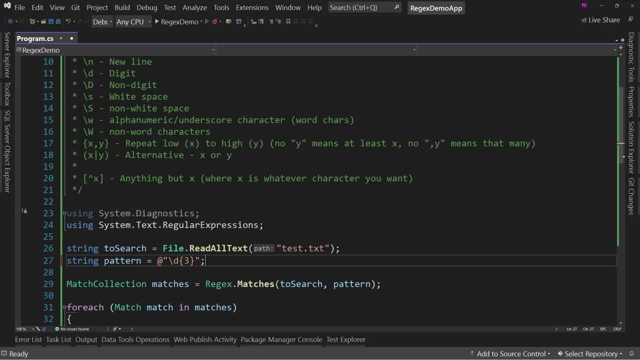 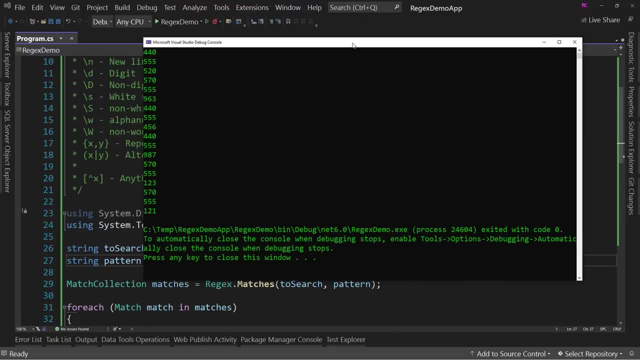 but if we drop the comma Y, see the difference there. if we drop the comma Y, that means that many. So I'm going to say three digits. I'm looking for specifically three digit patterns. Now if we run this, we'll see we have a number of three digit patterns. but that's not good. 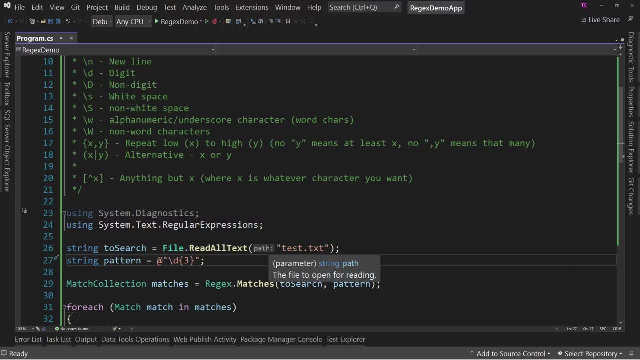 enough, because that's not the, that's not a complete phone number, That's just the first part. But then you want to say, okay, I want to have a another three digit pattern. Okay, I know a three digit pattern and 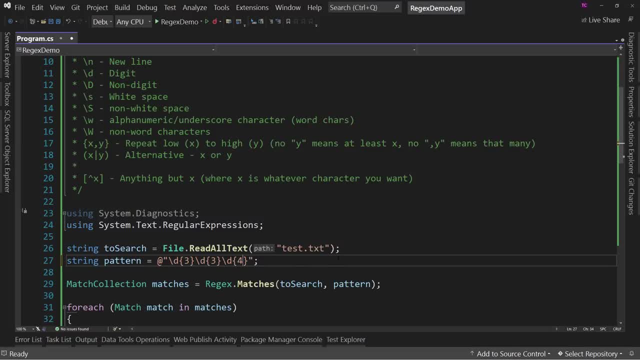 then a four digit pattern. So what this would, what this would find. let's just put a search here. This would find the four, four, oh five, five, five, one, two, one two or whatever the actual. 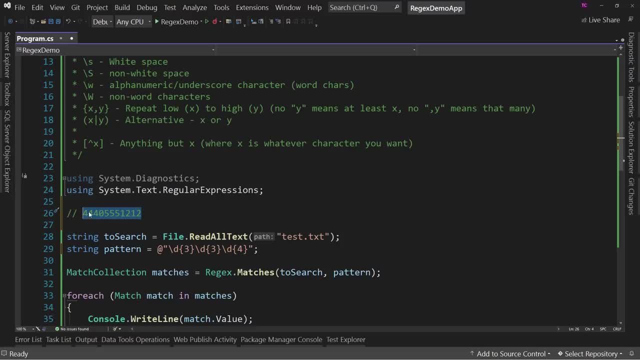 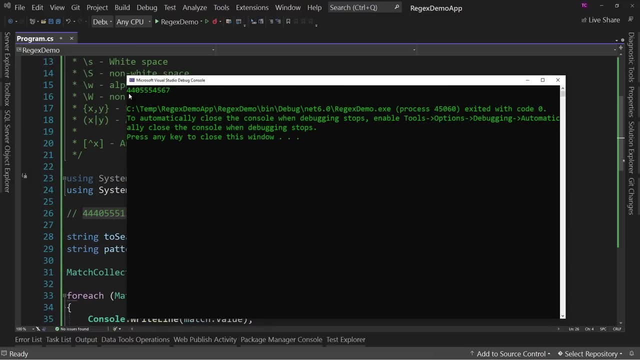 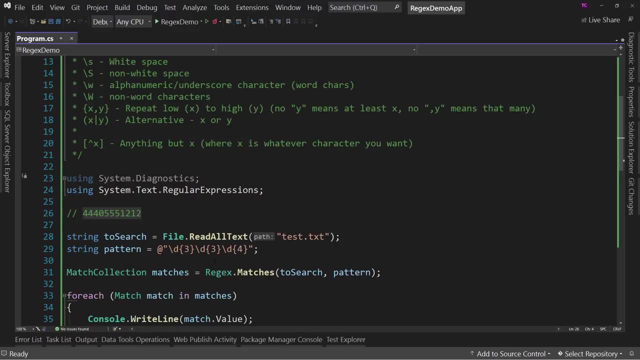 phone number is. That's what this would find. Now it could have just said digits of of 10 and find this. but let's run this And sure enough, it found just one, four, four, oh, five, five, five, four, five, six, seven. That's the one phone number that matched this pattern exactly. 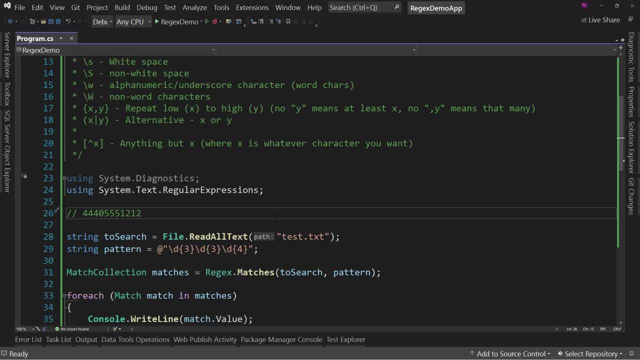 But we have options for phone numbers, For example, sometimes people oops, I have one, two, eight, four there. Sometimes people put the dashes in between. Well, let's handle that. So in between between our first three and our next three, we need to have a dash. So we're just going to say: 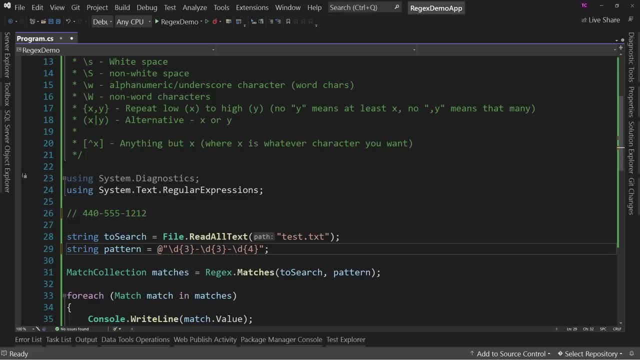 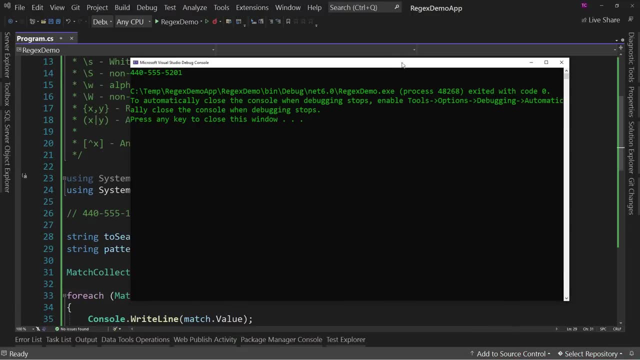 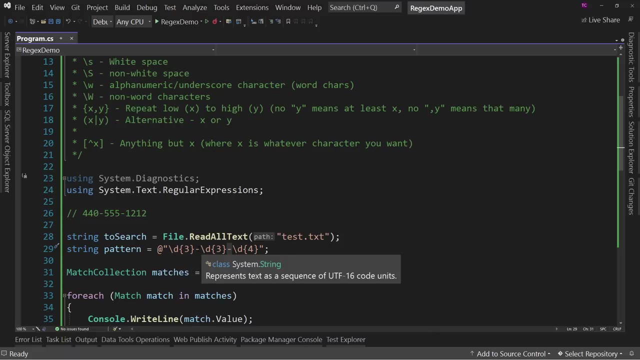 dash and we'll do dash between the next three, And this is a regular character, So it works just fine as a real character. If we run this, we found the one has dashes, but we didn't find the one we just found, because we don't always have dashes, And that's where this character 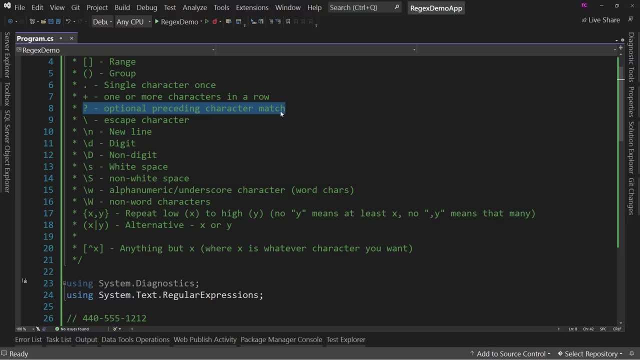 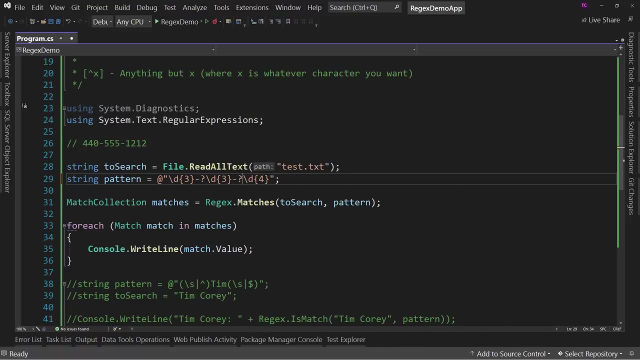 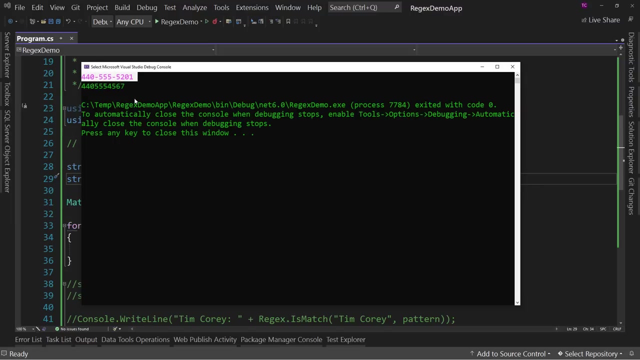 right here comes in. So let's run this again. And now we see two matching numbers. We found the one that has no dashes as well as the one that does have dashes. Now let's look at what else we could do. Well, 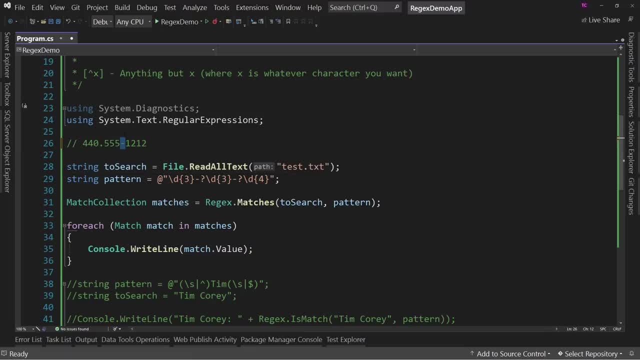 sometimes people will put. well, sometimes people will put the dot in place. So let's take care of the dot as well. We already have a dash in that place. How do we do a dot? Well, we can do the or. So it's either a dash or a dot. So if either of those is true, 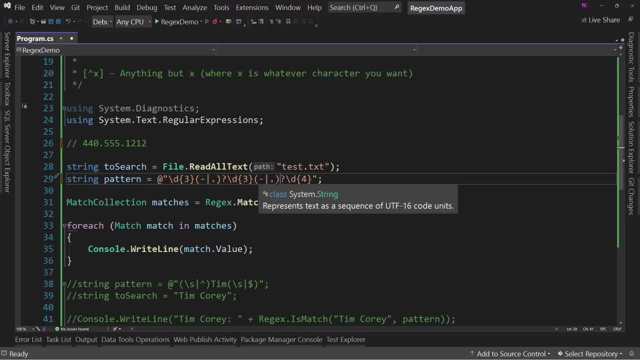 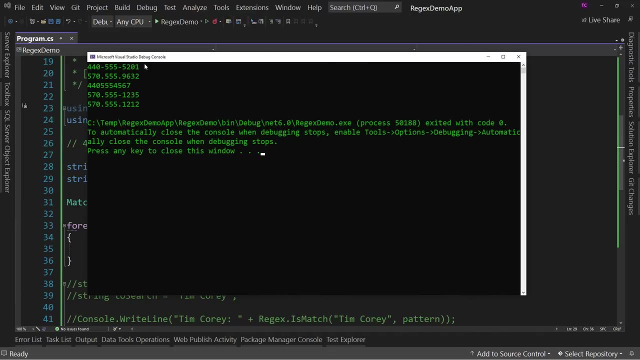 let's do this for over here as well. If it's either a dash or a dot and it's optional, is this optional? Now applies it everything inside the parentheses, So it can have nothing. It can have dashes, It can have dots. Let's run this again. And now we have five phone numbers. You have the dashes, We have. 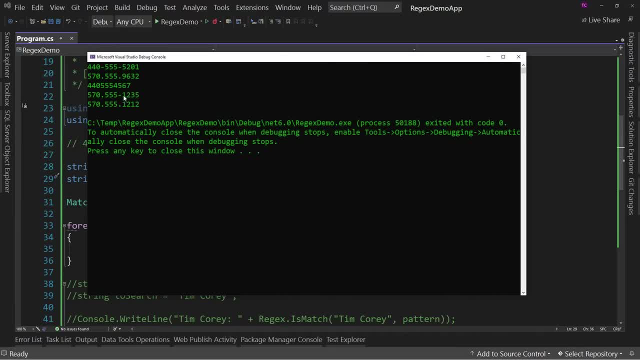 the dots. We have nothing. We have the one that has mixed dots and dashes, and we have the other one that has dots. So we've now found five different possibilities. We haven't found the sixth. So where do you find the sixth possibility? 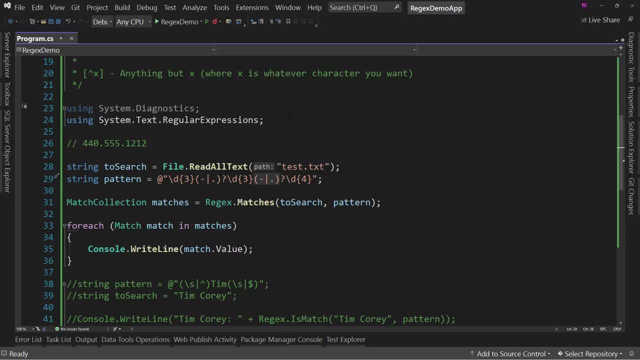 Well, we can look for the one that has this, And this is another way that. yes, we have a lot of different ways to create phone numbers right, This pattern where you have an open paren and a close paren and then you have a space- or not, but usually a space- and then you have a dash. 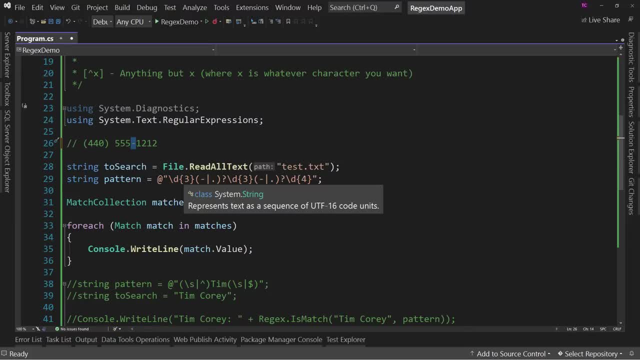 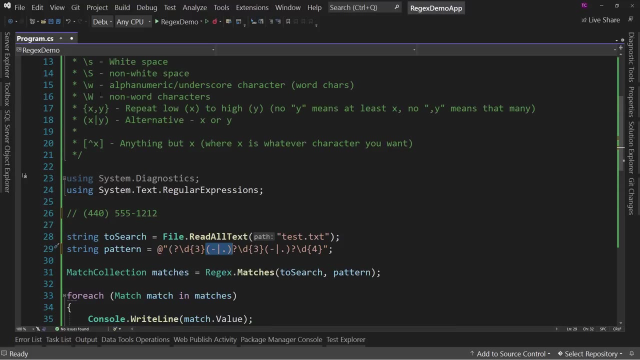 Well, in order to do that, we need to start off by looking for an optional, optional parentheses, So we can say: parentheses and a question mark meaning optional right? Well, not quite, because, remember, we use parentheses to say: to use this for an alternate. 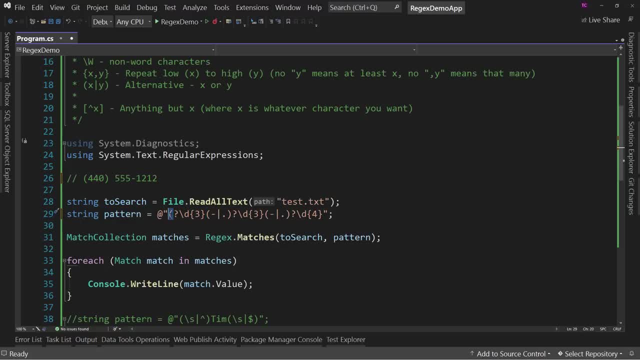 alternate. So how do we put an actual parentheses in here? We have to escape it. So now you've escaped that to say: no, this is just a parentheses, okay, So we're looking for this as a optional parentheses and then we'll have to look for an. 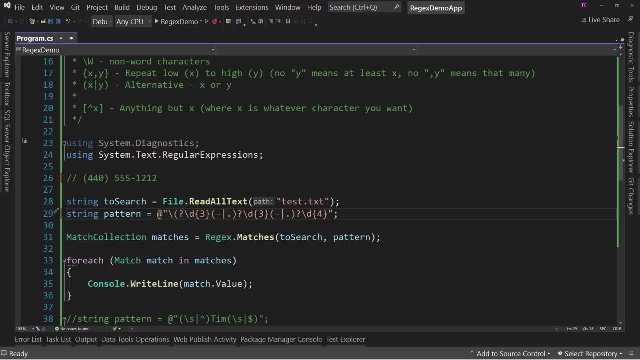 optional parentheses, All right. So we're going to say: slash parentheses to escape that parentheses, but that's optional, And then we could have a dash or a dot. We also have a space, So let's have another option here: slash S for space. Whoops, wrong slash. 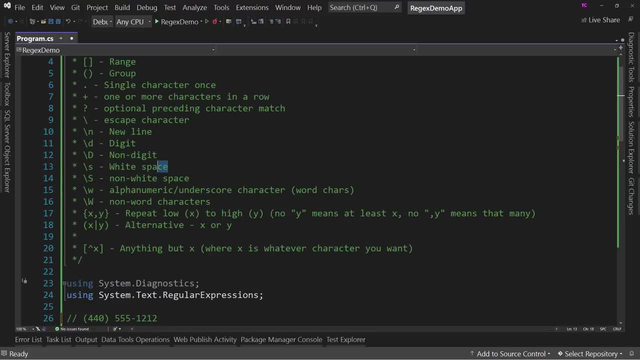 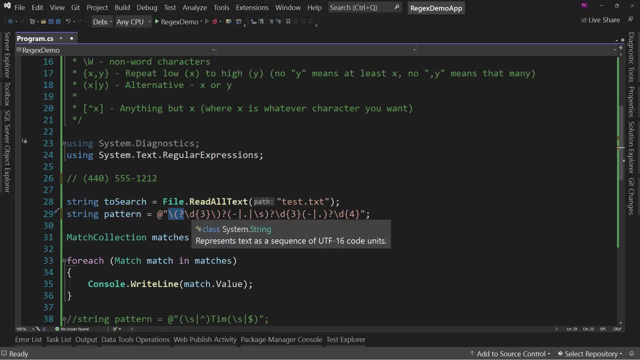 Slash S for space. Again, that's up here white space. So now we have a optional opening parentheses, We have our three digits, We have an optional closing parentheses and we have an optional space dot or dash. Now why didn't I just put? 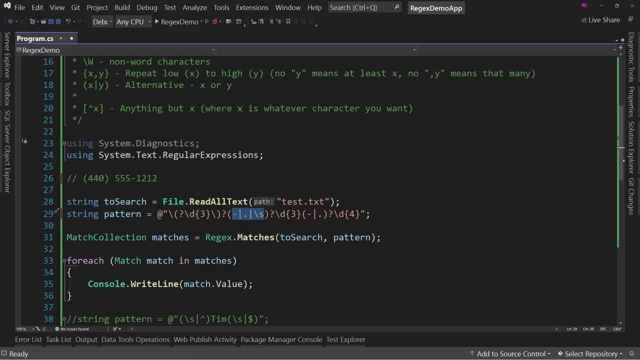 this inside of my set of ors. Well, because it's actually two characters that may or may not be there, So this is optional. but if we have this parentheses, we probably have a space as well. So that's where that or comes in. We don't have to, So that's why I've separated it out. 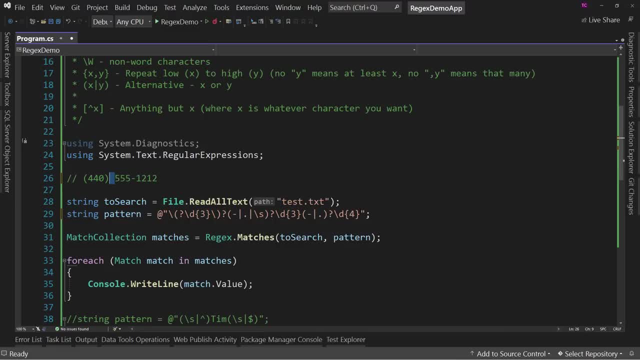 And yes, now we're starting to look like a very complicated statement. We've got all these slashes and squiggly brackets and question marks and dashes and dots and all the rest. We're saying, man, that looks complicated, But when we broke it down and figured 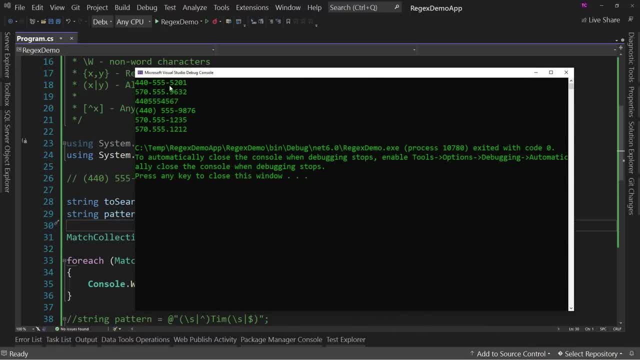 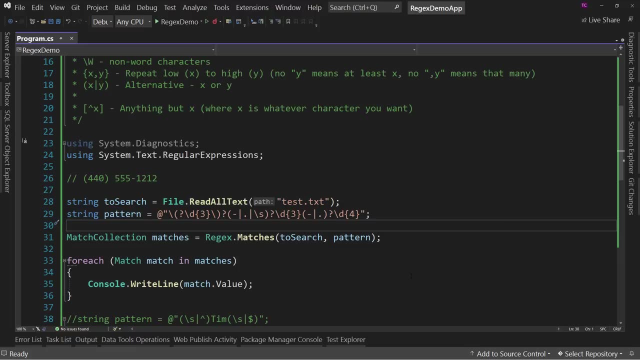 out what it does. it works great. We've now found the six phone numbers that I buried in that text file almost instantaneously. This thing is super fast, So that's why regular expressions are so powerful, If you decide you want to look up and find a phone number in this whole huge text file. 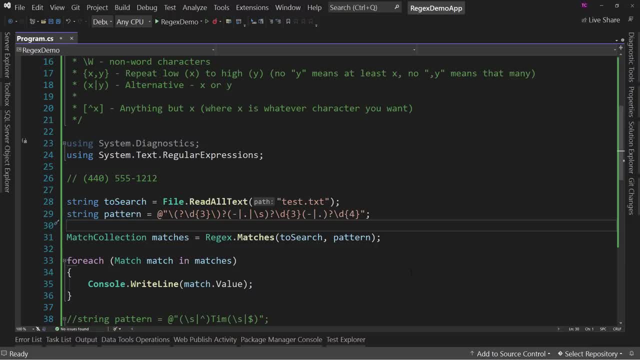 you think you know. I think they left me a phone number somewhere. There you go. Quick look up If you want to pull out certain patterns like an email address, or email addresses are hard, by the way, don't think you've got to conquer it. There's some complexity around an email address. 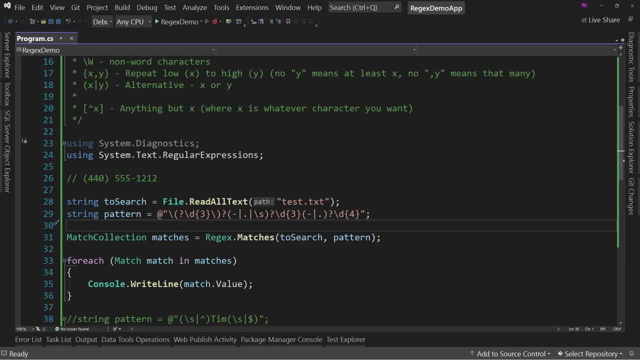 but phone numbers, zip codes, addresses, names, words- so many different things you can find using regular expressions And while the statements do start to become rather complicated, at least looking. when you start to break down, you'll notice that the text files are not exactly what they're doing in reading them. 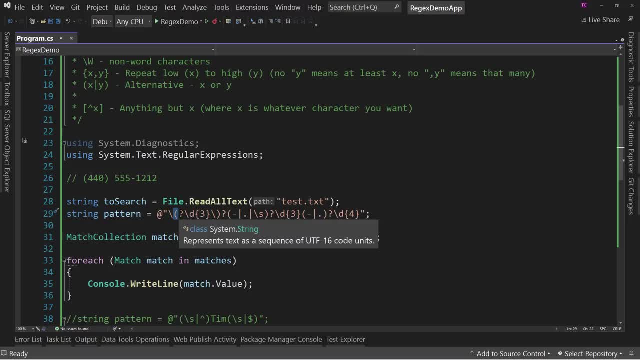 character by character or two characters at a time, Sometimes like, for example: okay, it's an escape character, What's it escaping a parentheses? So it's just a character, the parentheses character. This means the proceeding is optional, So that is optional. 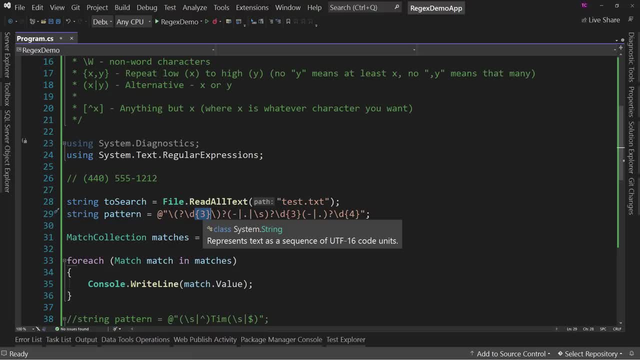 Okay, This means a digit, This means times three. So I'm looking for three digits with a possible parentheses after You start to read through this and go: wait, that's not that complicated, It's just. it looks ugly, It's not easily human readable, You don't just look. 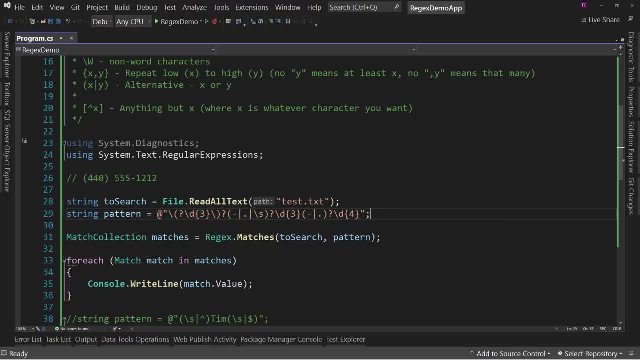 at it this- at a glance At least, I don't- and go: oh yeah, I was looking at phone numbers. That's hard to do, But when you start to slowly build it up over time, you create this complicated statement that does exactly what you're looking for Now. we could make this even. more complicated And we probably. okay, if I were to just read this one thing at a time, I think I'd have two minutes of information. I think I would have more than that, but you don't have to look at it. 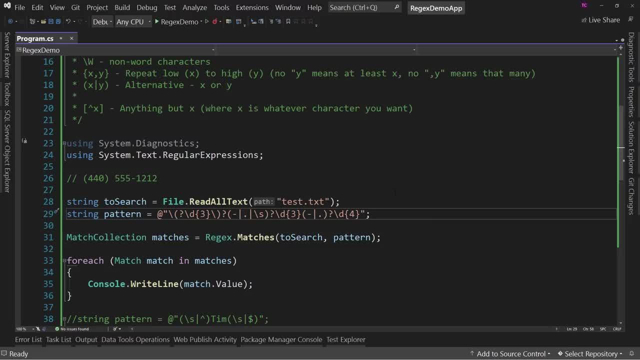 if i was going to create this for a customer, i probably would make it more complicated, and the reason why- and this is where you start to think through and use the logic you've been building as a c sharp developer- think through the edge cases. now it's found, all the ones i put in. 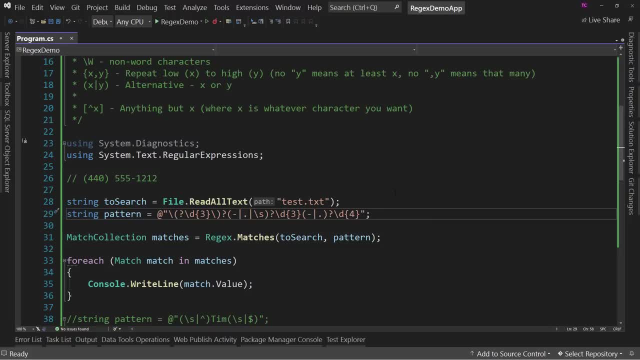 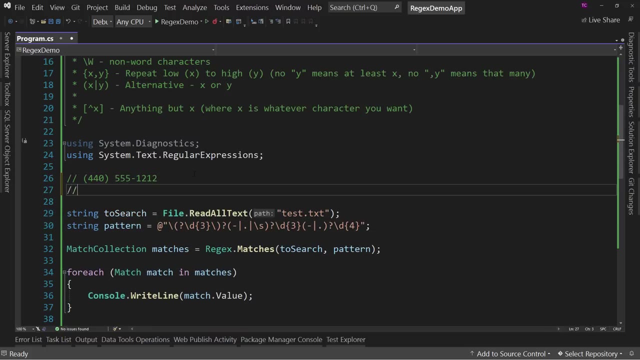 there, however, what it only has phone numbers in that file that are actually numeric. the rest aren't phone numbers. so i would throw in there a few other things that aren't phone numbers, maybe a um, maybe id code, for example, if we had, you know, uh, one, one, two, dash, three, four, five, six. 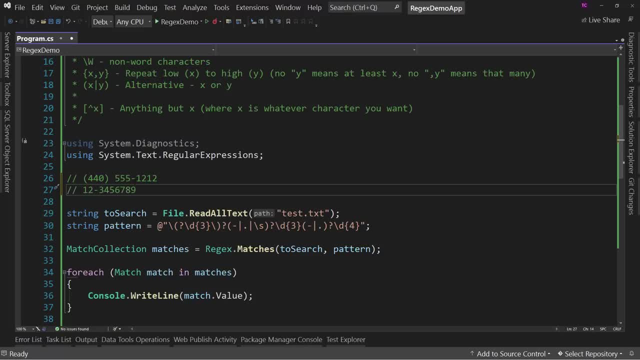 seven, eight, nine, um, uh, zero. that's technically 10 numbers. make sure that doesn't trigger a phone number. that's an id number, that's not a phone number. and then you have to think through what if we put the one plus, if you're in the c sharp developer and you're in the c sharp developer. 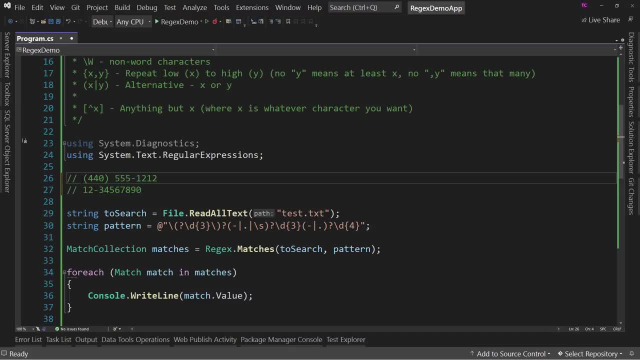 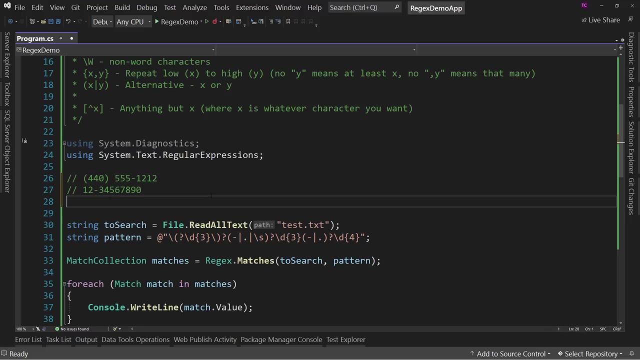 us. that's the country code. so you had you know, uh, or plus one like that- that we're not picking up the country code. so if it's a different country code, that'd be a problem. it doesn't work with international phone numbers. we think about that, um, do we think through things like: well, what if? 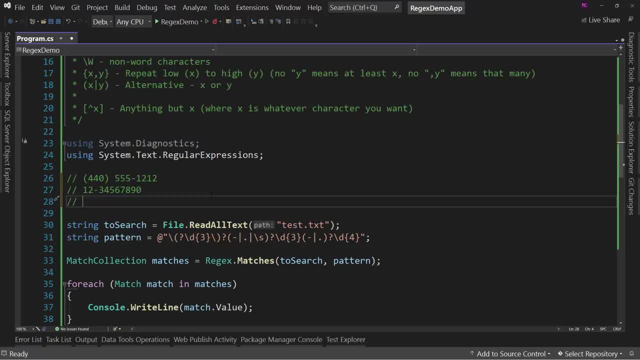 there is a um, i don't know. you know, if i were to say one, two, three and then we're gonna say something else. you know, maybe a zip code and i say like that is that can get triggered somehow by a phone number lookup and start throwing these edge cases out to see if you can figure out well. 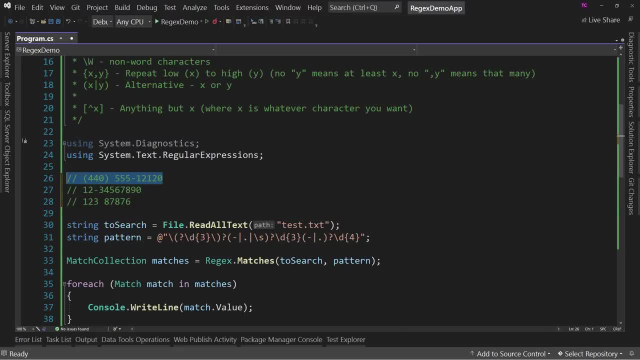 what if there's a you know, is that a phone number? no, it's not a phone number because it's not the right number of characters, but it would be picked up as a phone number because it found this and so this is a phone number. so i need to think through. okay, kind of like our name here, a. 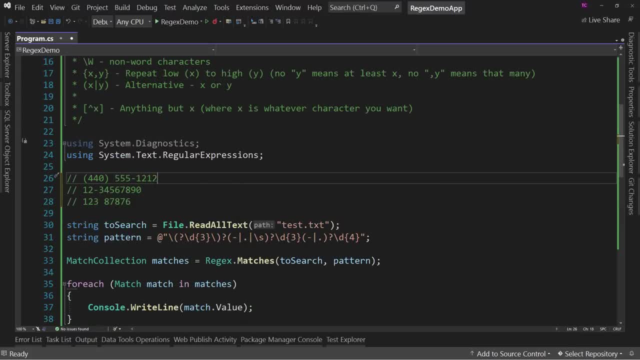 red screen. read the message: Eeny, Meeny and Meeny. I'll figure out here and what your is, brain number. if i'd just od, if i don't want toим is the same name, i'll have to add two different addresses of x and y. i'll have to type in my name. it's something up here, so i need to move. 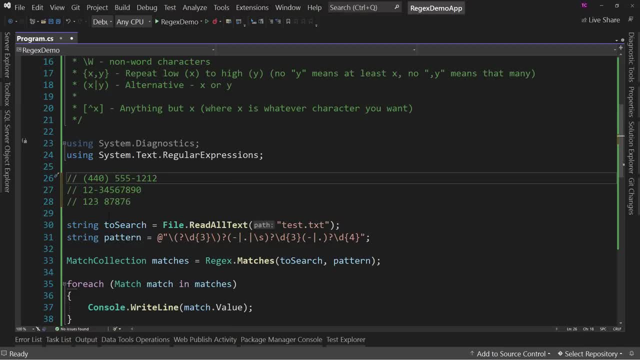 these governs, but that's what mySIX2006C над dynamics is. um, i'm going to count these out, so i'm gonna put a one よ. Okay, So these are super useful in certain circumstances, Now that you know how to use. 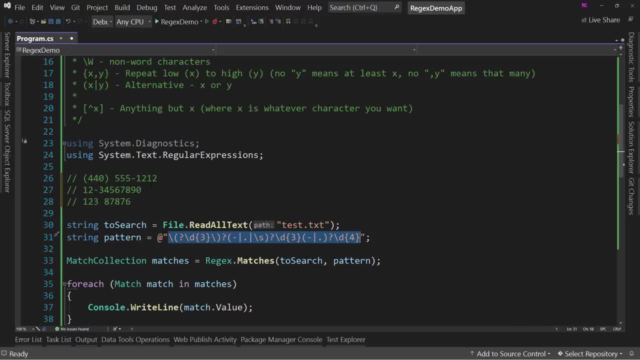 a weather expression. don't look at every lookup problem or query problem as a option to use weather expressions. Okay, Make sure that the solution fits the problem. This is a tool. It is not meant to replace every other tool you have. Use it when it's wise to do so. 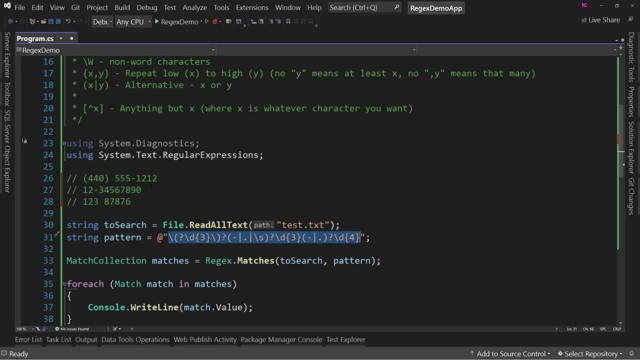 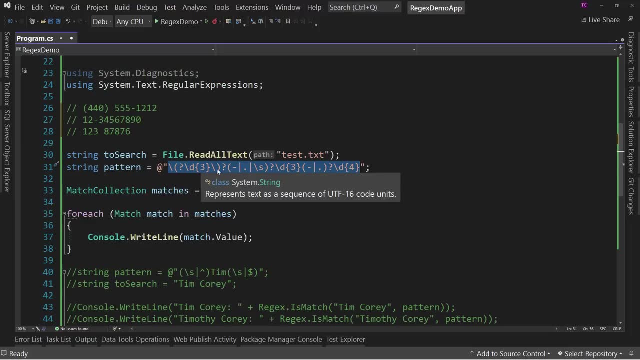 when this is the best option. If it's another option that is simpler, use the simpler option, because when you're scanning through your code, that's kind of a road or a speed bump. Okay, Remember, I've said a number of times that source code is meant to be read by humans. 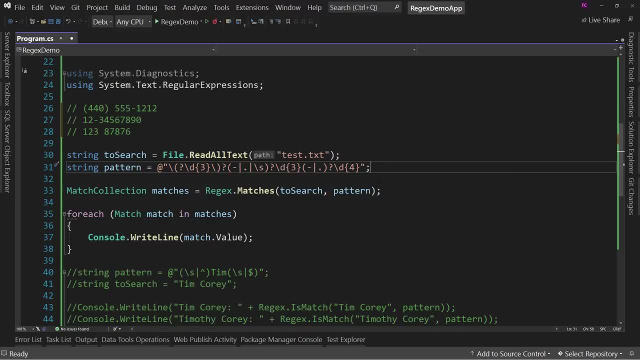 not computers, humans. That's what's meant to be read by Now. computers do read it and they do compile it. But remember, computers compile things down to ones and zeros. We don't read ones and zeros, We read C-sharp code. 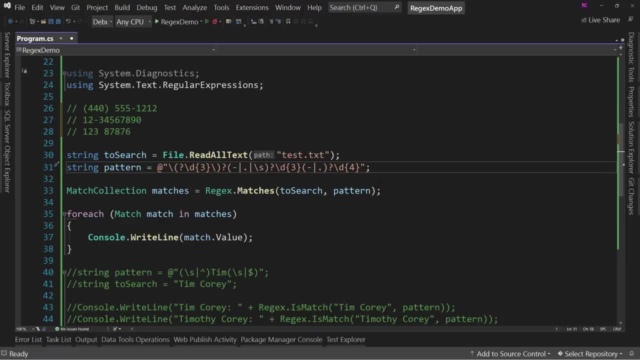 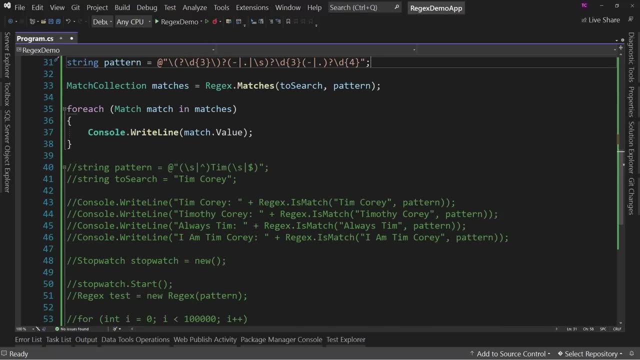 And that's why it's meant to be read by humans, because we're going to be the ones debugging it, We're the ones that try to understand it and to improve it, And so when you read down through source code, it's very easy to read right: Consolewriteline. Okay, That's writing to. 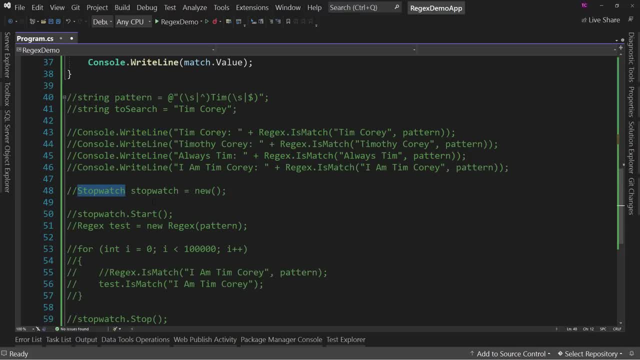 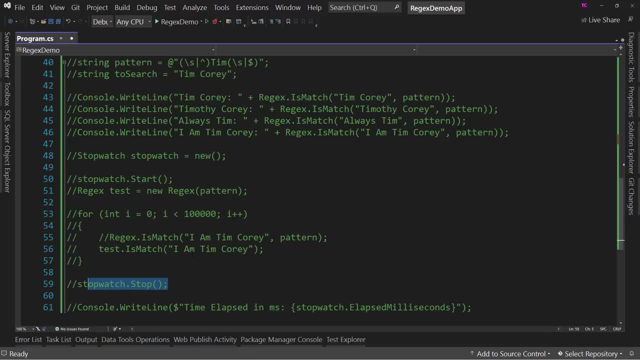 the console: Cool Stopwatch. Okay, I understand why Stopwatch is stopwatchstart. I got that Stopwatchstop. I got that. Even if you didn't know about the stopwatch class before this video, you probably have a pretty good grasp on what it's. 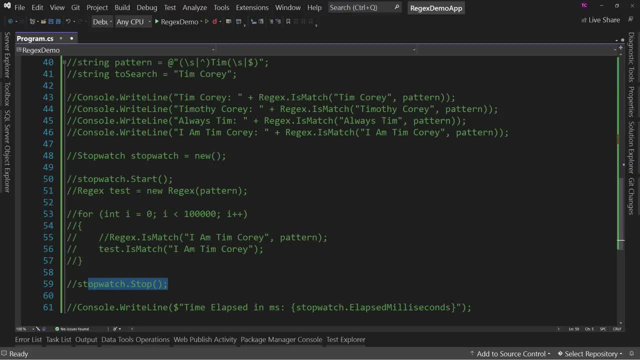 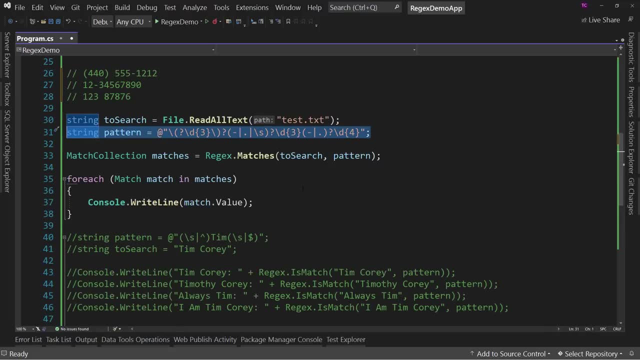 doing. It's starting and stopping a stopwatch. That's human readable code. When you get to a expression and you see pattern and you see that you go. I have no clue And so you have to stop- You're reading, your you're using and say, okay, what is this doing? And you start one character at a time And if 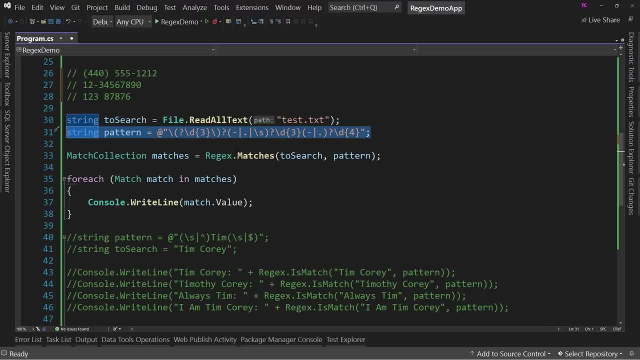 you're like me, maybe you're not, maybe maybe you look at regular expressions and go: man, I got it. That's, that's super simple. That's a, that's a. you know, that's a phone number. 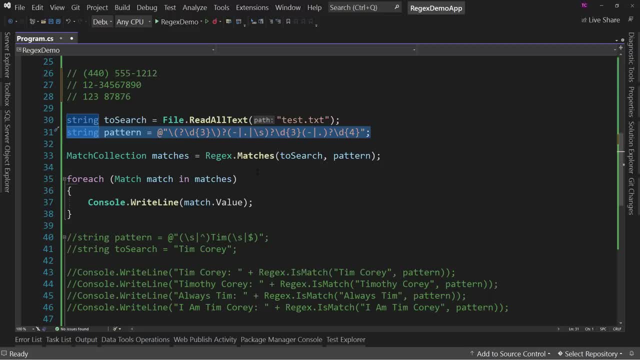 No problem, I see the three, three, four pattern and the question mark Got it. But for me I have to go through and read character by character and write things out and and kind of figure things out. It takes me a long time sometimes to figure out what a regular 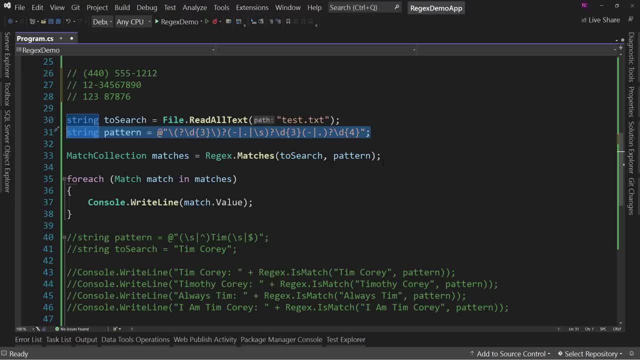 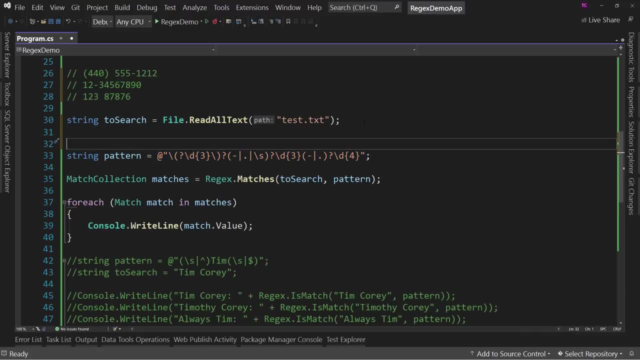 expression is: Is doing or trying to do one thing would help, And I highly encourage this. People say some people say that you should never have code comments. That's wrong. That's just wrong. Whenever you say never in programming, you've probably made a mistake, because if you go to an 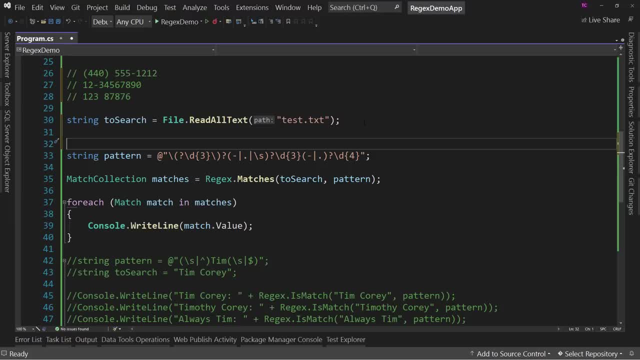 extreme, always or never, then you are leaving out any possibility for an edge case, And life is full of edge cases. If you speak English, you know there are tons of edge cases in our language itself. So edge cases are a thing because the world is unique. It's not like we fit into the same pattern all the time. 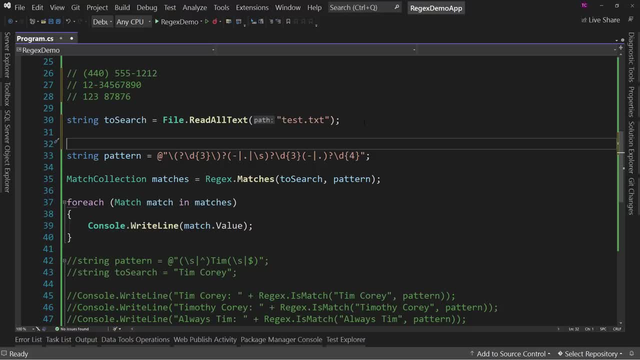 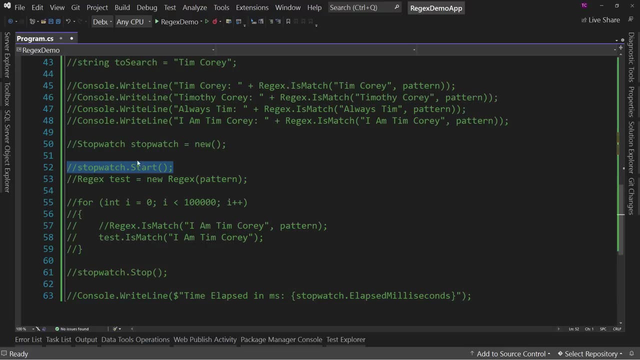 Otherwise we wouldn't need software developers. We would have solved every single problem because it would have all been known. but no, we have edge cases. So, when it comes to code comments, I don't recommend commenting things like the stopwatch, not start. That's pretty obvious what it's doing. That's code that you can easily understand. 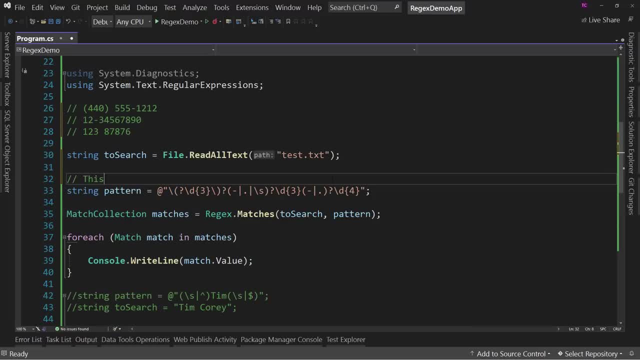 But this, I would say: this pattern matches phone numbers, And I might even say in the following patterns and specify them. Okay, The only thing is- and this is where the the no code comments people have a good point- is that if you come back and say, oh, we need to. 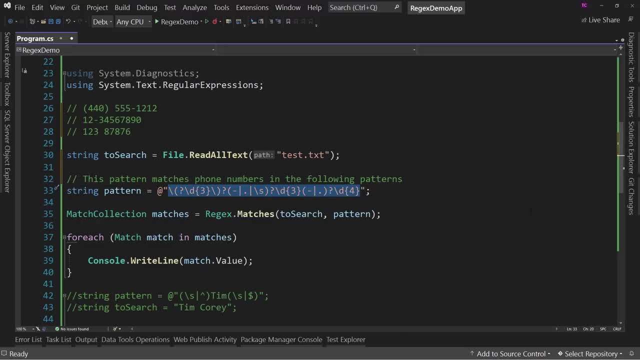 adjust this to also take into account the idea of people using- I don't know- commas instead of periods as well. Okay, Well, you need to update your code comment as well, because otherwise your code comment is out of date, And it's actually worse than not having a code comment sometimes. 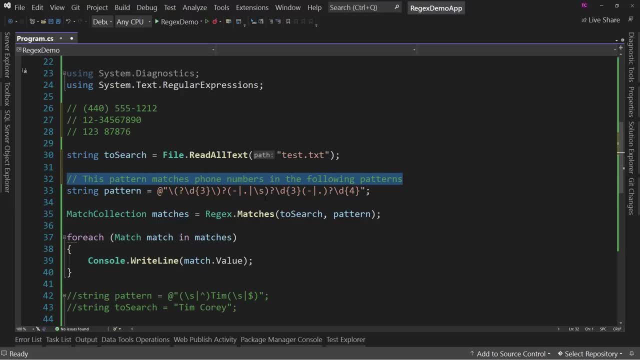 because the code comment is what's easily readable And some people read that and believe it, And if it doesn't match what's actually happening, that's a problem. So if you do have a comment, you have to maintain it, Otherwise it's actually worse than not having one. 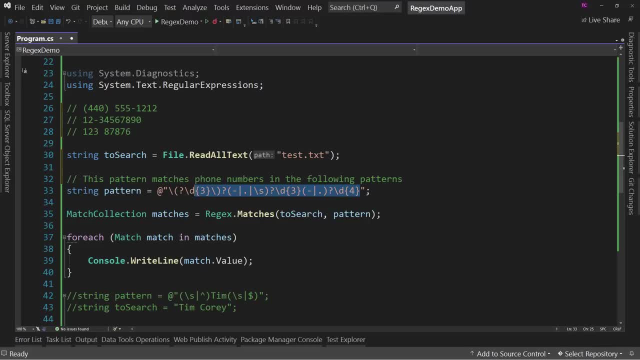 But in cases like this, it's important to have a comment to make it easier for people that are scanning your code that don't necessarily need to handle updating a pattern because maybe they're just looking for another part in this, this section. They don't need to understand everything that that is doing, They just need to know.